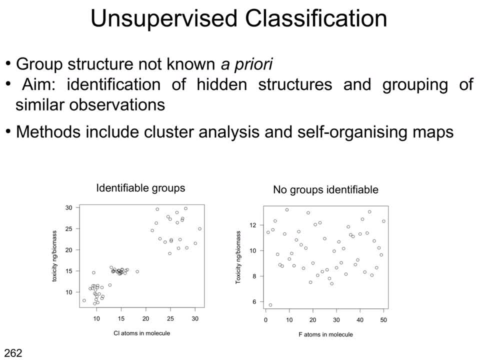 On the left hand side we see that we have identifiable groups. We have the chloride atoms in the molecule against the toxicity pro-nanogram biomass of animals And we can see that when chloride atoms are added to the molecule That you have some stepwise jump in the toxicity. 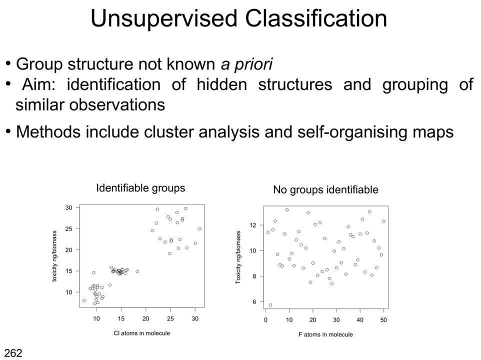 So toxicity is relatively similar between 8 and 11 molecules. Then it jumps when you have about 13 up to a higher level of toxicity. That remains more or less the same, And then, once you reach 22 molecules of chloride in atoms, of chloride, in the molecule, in the complete substance. 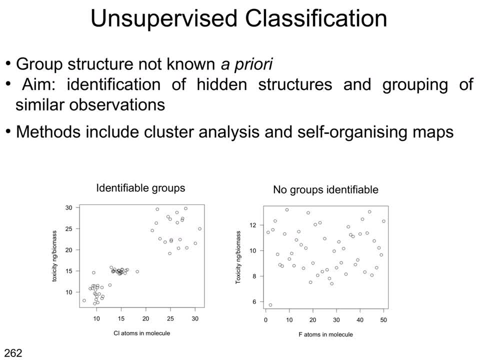 Then toxicity increases to a new level In the right figure we see that we have for fluoride atoms. We see no relationship between the atoms in the molecule and the toxicity And we couldn't identify any groups in this case. Overall unsupervised classification methods. 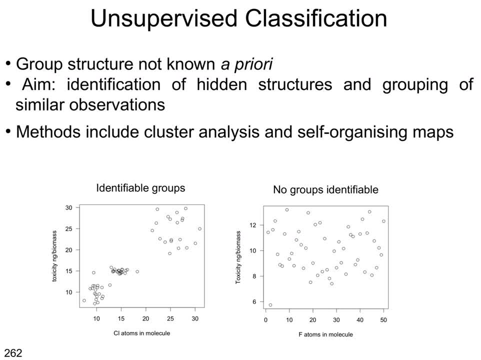 Have been developed for different purposes And there are different methods available. One of the most prominent methods is cluster analysis. That has a longer history than many other of the novel methods. Novel methods include, for example, self-organizing maps, But we limit our discussion to cluster analysis. 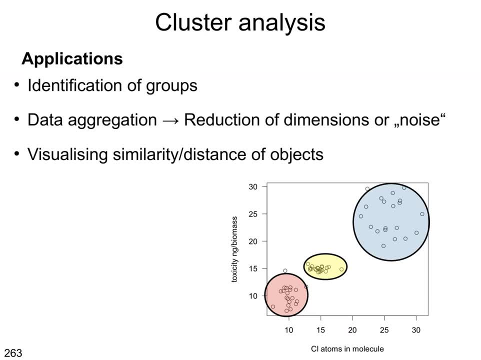 So cluster analysis has many applications. One of the applications we have already discussed: It is used to identify groups. That's not surprisingly. That's the aim of unsupervised classification, One of the main aims, And, for example, we could look for groups of plants. 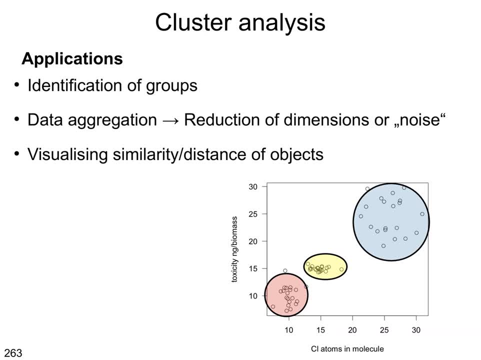 That have some similar characteristics But are different in these characteristics to other organisms Or other objects of the same type, For example, plants that grow very much, And we want to distinguish them from plants that are slow growing Or animals that are herbivores. 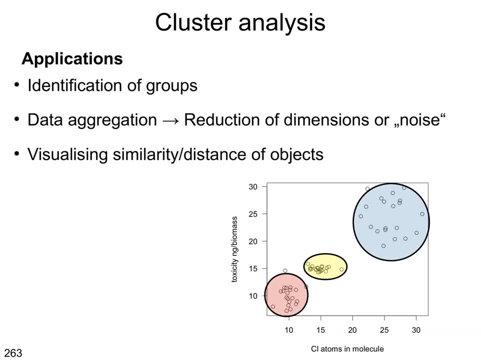 And we want to distinguish them from omnivores and predators Or parasites. We could also look at genes And try to identify genes with a similar expression patterns. Cluster analysis is actually used in all these contexts. Then it can be used for data aggregation. 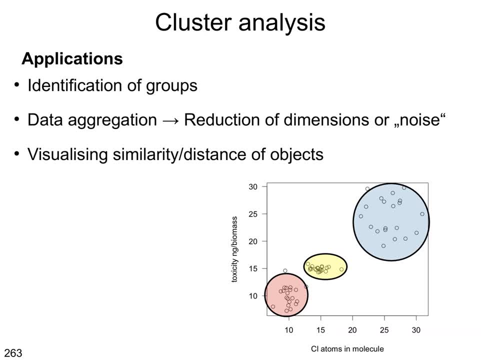 For example, if we want to reduce the noise in the data set, We can replace the individual observations in the data by the group centroid. So if you look at the circles or the ellipses That we have created on the figure- The blue, yellow and red- 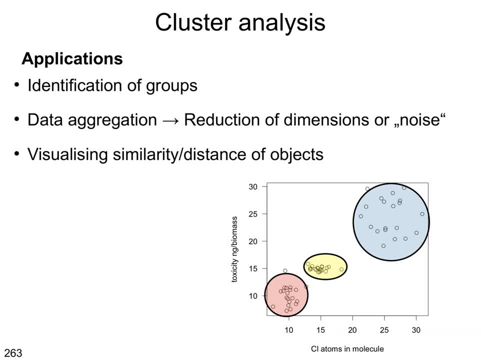 You could replace the individual observations by just the mean By the center of these data And use that in subsequent analysis. You lose some sample size, But you gain some more. You reduce the noise in the data. In addition, we will show you. 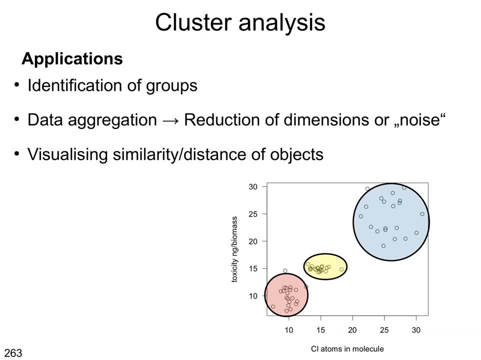 That through cluster analysis You can reduce the dimensions of the data, For example in the dendrogram. This dendrogram is also a way to visualize The distances or similarities between objects in a two dimensional space, And this is very helpful And an alternative to ordination. 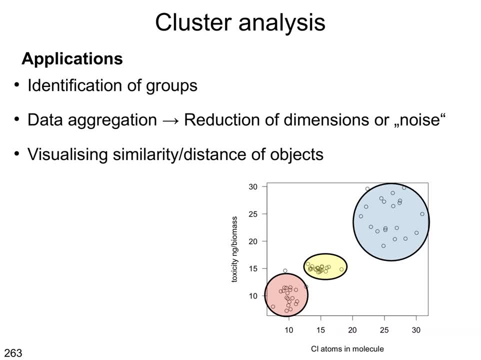 In case that we have really grouping structure in the data. Finally, we could use cluster analysis To identify outliers, For example, if we establish groups And we see that some of the points Deviate strongly from each of the other groups Or clusters that have been developed or established. 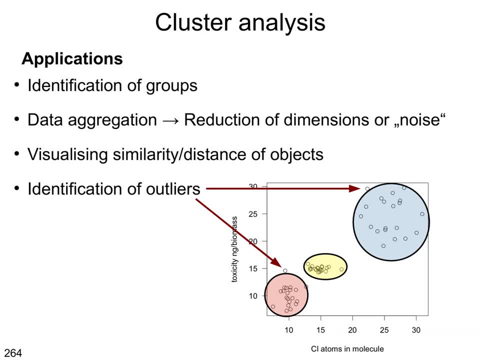 Then we could treat these points As outliers in the data set. In the notes to the slide You will find some literature hints Where you could look for additional material To read about cluster analysis For ecological data, For example Wildey 2010.. 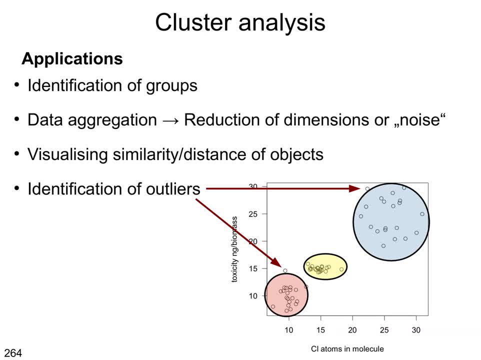 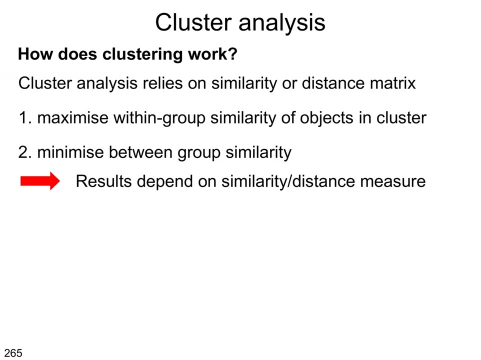 Or a modern treatment of cluster analysis, Is provided in Everett et al 2011.. You will also find this textbook On the literature list related to this course. So how does cluster analysis work? Cluster analysis relies on the similarity Or distance matrix. 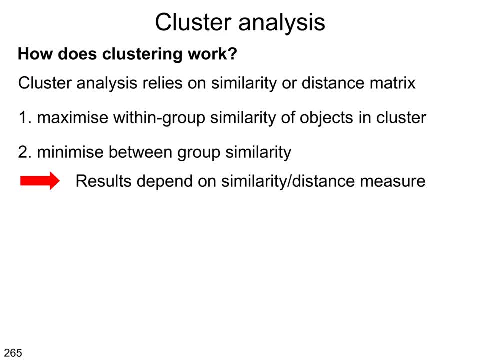 We have discussed different distance measures In the previous session, So you should be acquainted with that- And you want to maximize the within group similarity Of objects in the cluster Or, at the same time, To minimize the between group similarity, So to have clusters that are. 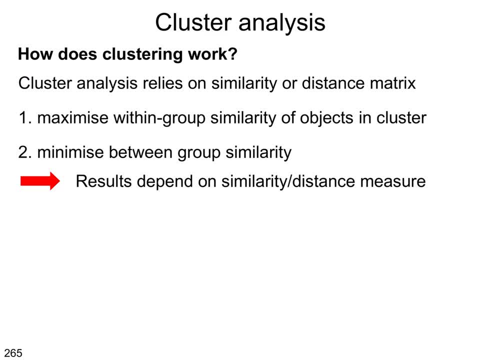 On the one hand, very homogeneous And, on the other hand, Are separated very well From other groups or clusters, And these results depend On the similarity or distance measure That is used, And that is actually the main problem Of cluster analysis. 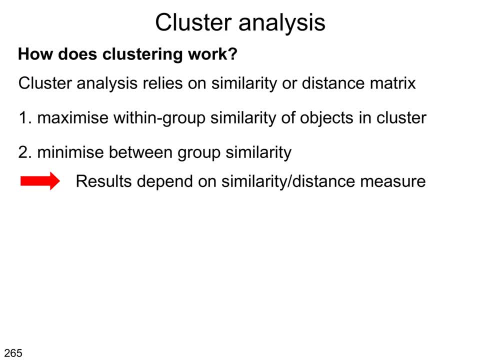 Because you need Not only to calculate similarity Or distance between objects. That is quite handy. We have done that, Although you know That there is a wide range Of different distance measures Or similarity measures That could be used And, obviously, the choice of these measures. 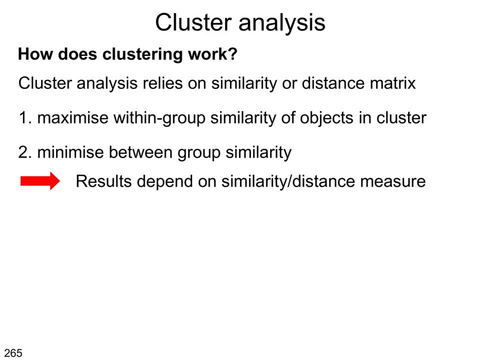 Influences the results, But we also need Somehow to calculate The distance between objects And the cluster itself, And how this is done Is discussed In a few minutes. We have Several different Types of cluster analysis, And we will first start. 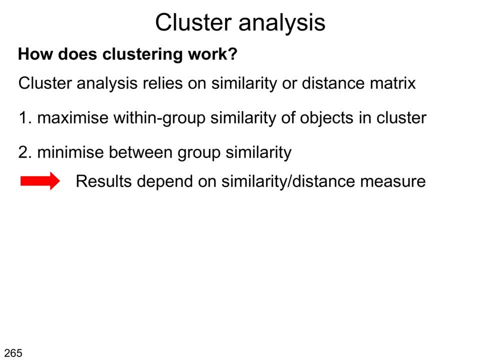 With hierarchical Acclomerative clustering. Hierarchical Acclomerative clustering Is widely used In many different fields of science. It is called Acclomerative Because it is Acclomerating the individual Objects with each step. 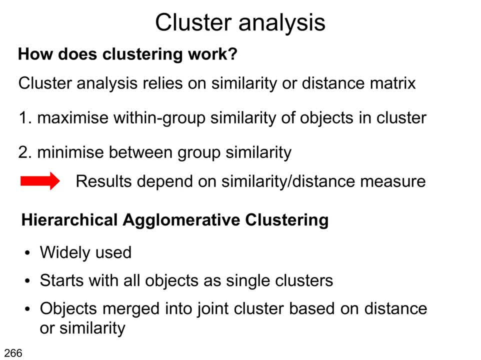 So if you have, for example, Different species Where you want to find feeding groups, Then in each step Of this cluster analysis, Two species Are merged together And form a new cluster And subsequently This cluster may have An additional species added. 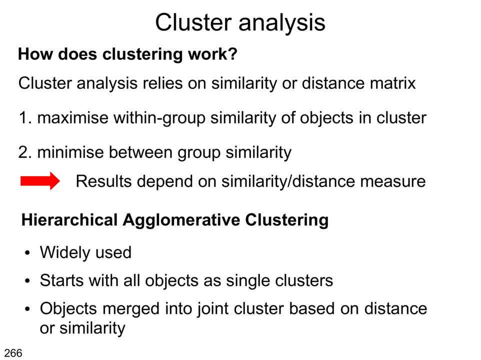 So in the end of this clustering All species are part Of the same Or have been assigned To a cluster And In the hierarchical Divisive clustering Would be the opposite. It starts with one big group And breaks smaller groups. 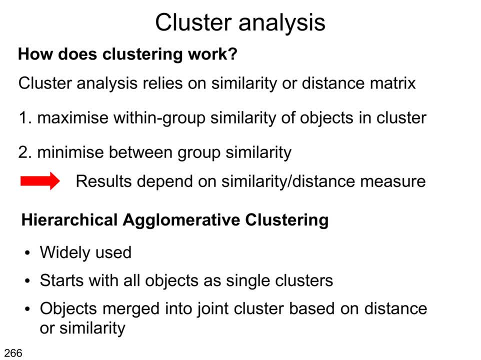 Out of that In each step So it breaks apart Smaller clusters from that. So this may be useful If you are searching for outliers, Because outliers form their own group In the At first In this kind of analysis. 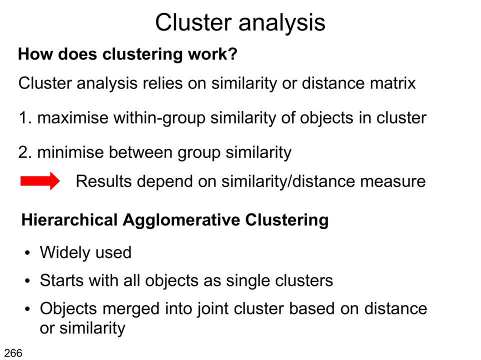 So in hierarchical Acclomerative clustering We start with all objects And then they are merged Into a joint cluster Based on the distance Or similarity. And how this is done exactly We will discuss now. So how does hierarchical 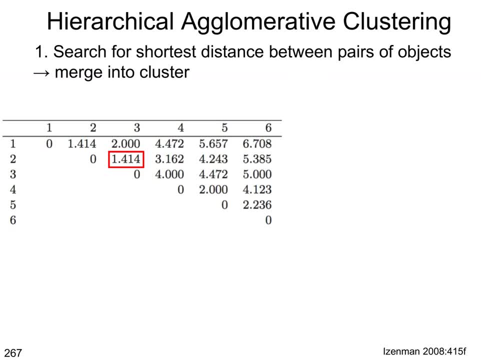 Acclomerative clustering work. We show you an example Here of some data Where we have produced A distance matrix That is displayed here. We have six different Sites And some characteristics Have been measured. And then, for example, 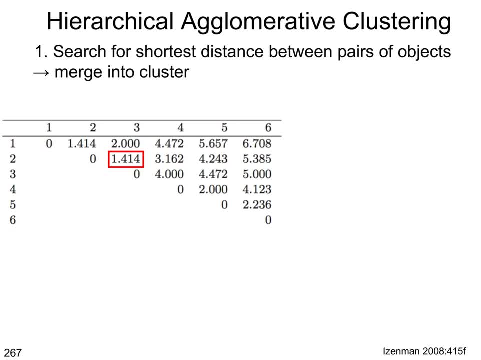 Some species Or environmental variables Such as the temperature or pH, And we calculated The distance Between them Based on the Euclidean distance Or, for species, On the Bray Curtis distance, And we see here The given distances. We do in cluster analysis. 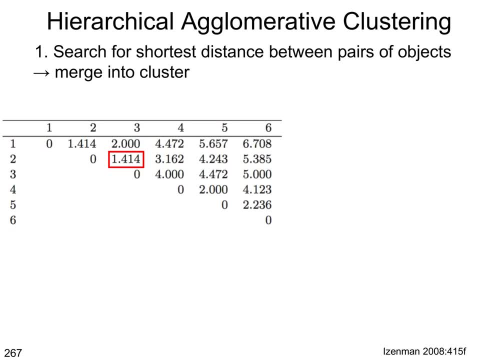 We first search For the shortest distance Between two objects, Generally in cluster analysis In hierarchical Acclomerative clustering, And we merge these two Pairs of objects Into a cluster. If we look at the distances Here of the matrix, 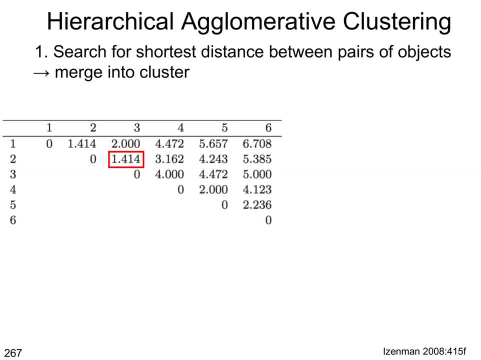 We see that one and two And two and three Have the shortest distances. Then, rather random, Whether you merge two and three Or one and two, There may also be additional digits Of the distances Where these two Can be discriminated. 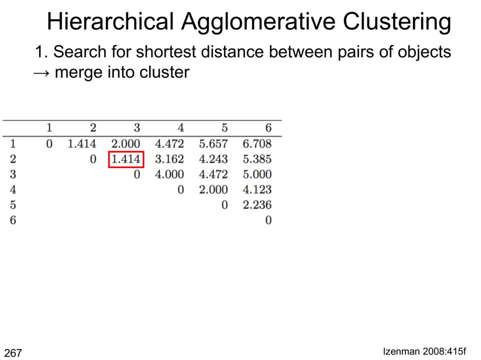 We see that Two and four, Two and five, Two and six Have higher distances, And three and four, Three and five, Three and six. What we now do Is we merge Two and three Into one cluster, Now that we have created. 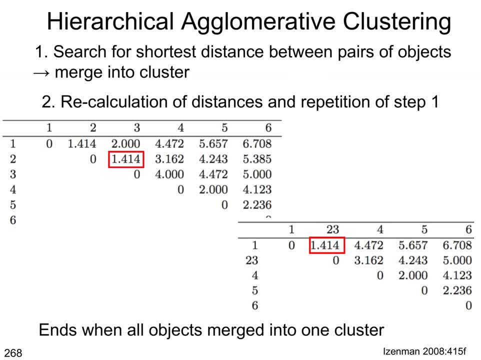 A new cluster. We see that we only have Five objects In our headers For the columns And for the rows, So we have one, Two and three, And we have four, Five and six. And now this is the challenge. 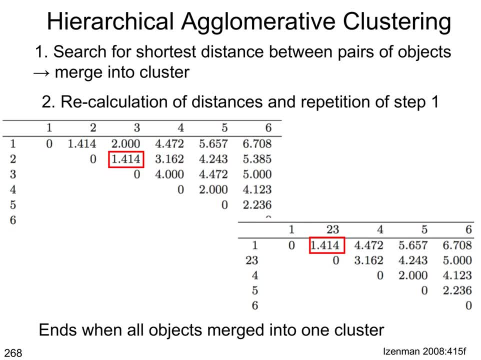 That I mentioned. How do we now calculate The distance between The cluster two and three And the individual objects One, four, five and six? Well, if you look at the initial Distance matrix, We see that, for example, To the object. 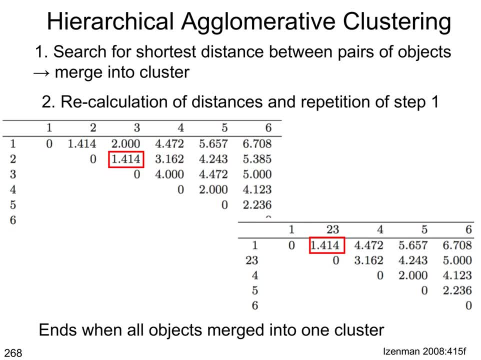 To the side one And side three Had a distance of two. So what is the distance of two and three After merging? We see here That the distance is one point four, And it's not difficult to identify That this is the lowest distance. 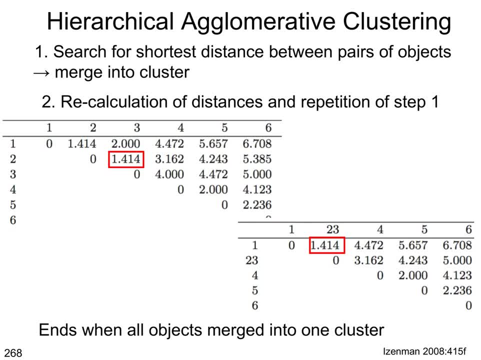 Of the two individual distances, So of two and three. We could go on And check this for other observations. For example, The distance of two And six Was one point three. The distance of Three and six Was five. 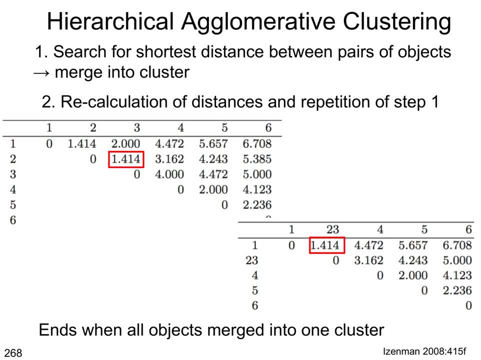 Now, the distance of two and three Is the lower one of these two. It is five. So what you do is You recalculate the distances And then You go back to step one. That means You search for the shortest distance. 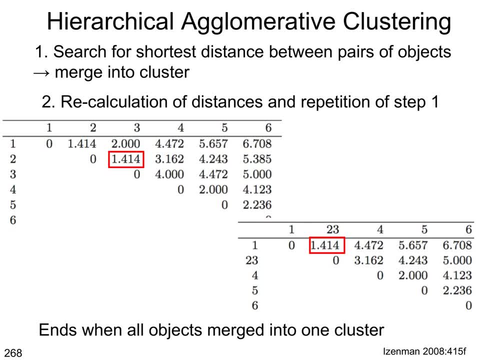 Between pairs of objects To an additional cluster. So what you would see here Is the shortest distance Of two and three Is the one, Is the distance To the side one. So we would merge The cluster two and three. 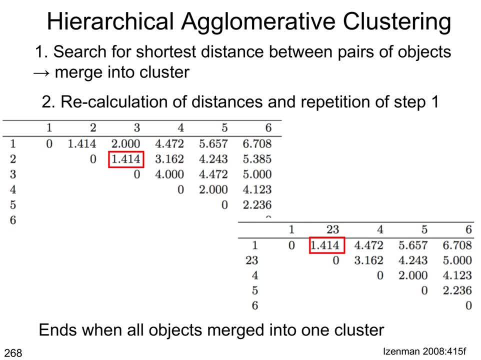 With side one, But in other circumstances. For other cases It could also be that, for example, Object four and five Would be closest, So we would form an additional Cluster, four and five- And we had Another grouping Then two and three. 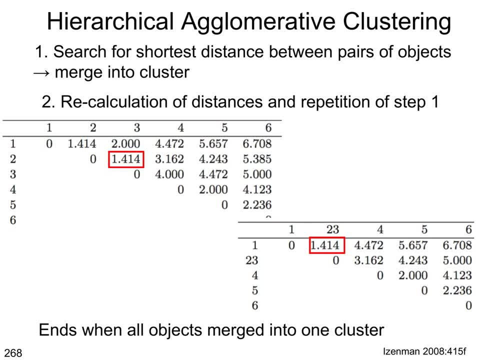 And we would need To calculate the distance between The cluster two, three And the cluster four, five. And this all, And this whole stepwise procedure, Ends when all objects Are merged into one Cluster, And this is displayed here. 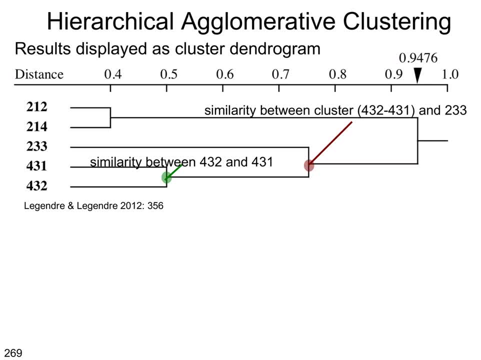 What is meant by that. It may be counterintuitive At the beginning That all objects Are merged into one cluster, But see what we mean By this hierarchical Agglomerative clustering. We have stepwise clustering, So in each step. 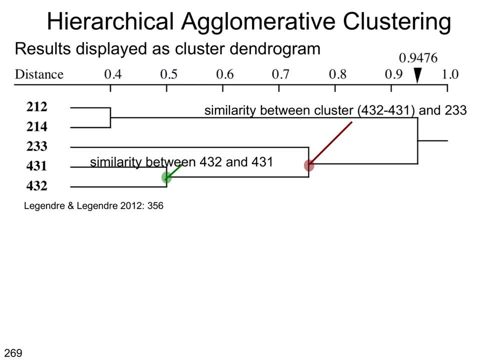 Two objects are merged. So have a look At this figure. So what we see, Say again, five sides, Two, one, two, Two hundred fourteen, Two hundred thirty three, And so on, And the distance between the sides Are on the x-axis. 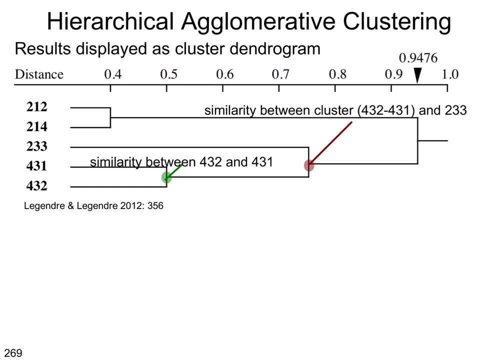 Now the two Sides, Two hundred twelve And two hundred fourteen, Seem to be closest, So they are merged first. Then we go the next step Where four hundred thirty one, Then we merge Two hundred thirty three With the cluster. 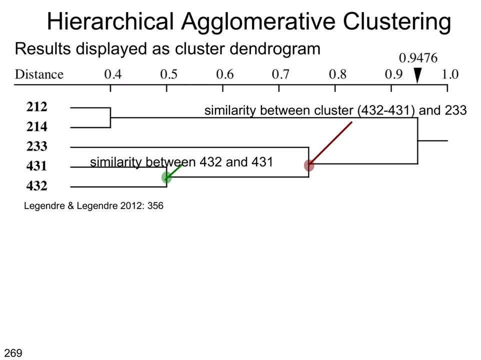 Four hundred thirty two And four hundred thirty one. Again, keep in mind That we are not looking at the distance Between two hundred thirty three And each of the individual points, But between the cluster. Four hundred thirty two, Four hundred thirty one. 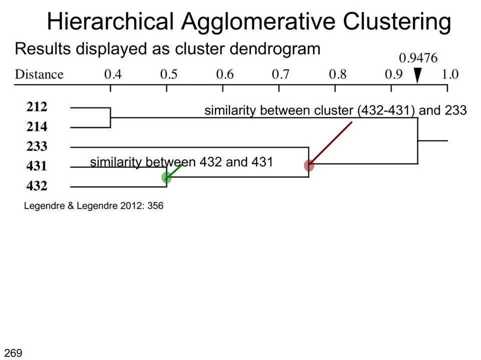 And after We have done this, We merge this cluster Of the three points now Four hundred thirty two, Four hundred thirty one And two hundred thirty three, With our first cluster. Two hundred twelve, Two hundred fourteen, And now all objects are. 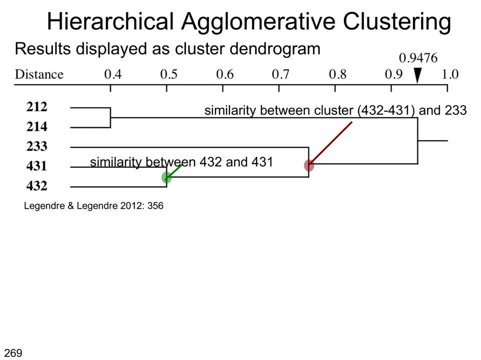 Are merged into one big cluster, And you can see The distance is almost one That means Between the cluster: Two hundred twelve, Two hundred fourteen, And this is the Similarity. So Note the similarity In the interpretation. 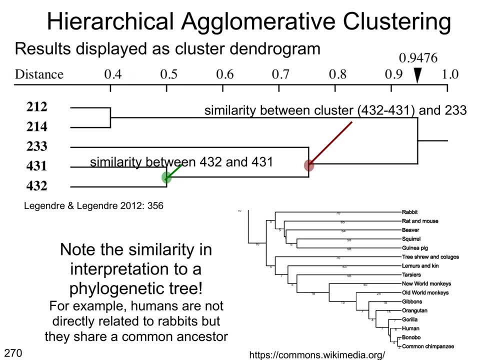 To a phylogenetic tree In a phylogenetic tree. Here you have The time on the x-axis Against The development of New organisms. We see That many of the primates And some rodents share a similar ancestor, so they have been merged. so if you move from right to left, 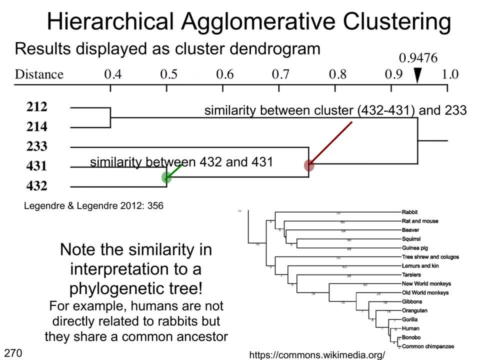 they all are merged and in the end they are having a common ancestor. so rabbits and humans share a common ancestor, but the similarity is of course not between- if you move along, that is not between the guinea pig and humans directly, but between ancestors that have been, that have. 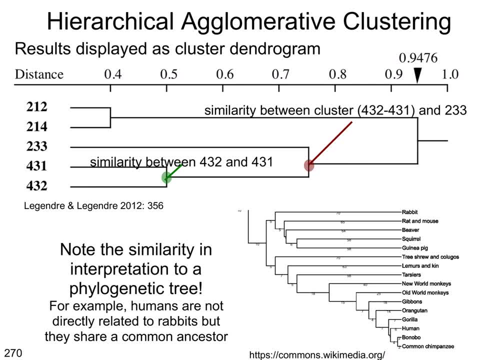 been living throughout evolutionary history and from these ancestors you have breakups of new species and that's very similar to cluster analysis, where we don't look. for example, when we, when we look at the joint well, ancestors For humans and rabbits, we need to look at the similarities between the whole. 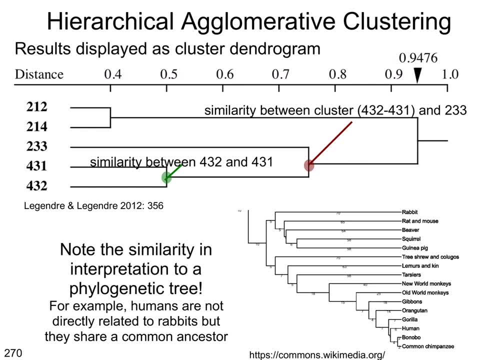 cluster of some primates and monkeys and some rodents. That's not the direct similarity between the humans and the guinea pigs or between the rabbits, And that's a similar interpretation may help to keep in mind what we have discussed about the cluster dendrogram. 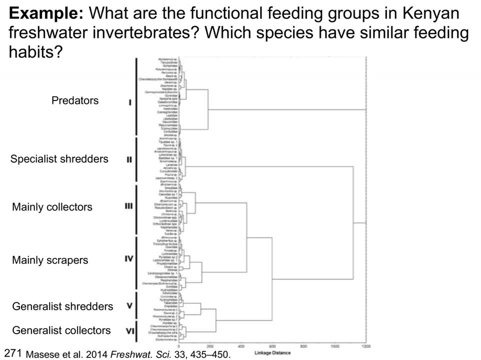 And here's an example from a study where hierarchical agglomerative clustering has been applied. The question has been: what are the functional feeding groups in Kenyan freshwater invertebrates? So many streams were sampled, the organisms identified and afterwards they used the different species Better. the characteristics of the species was the gut content. Here they looked. 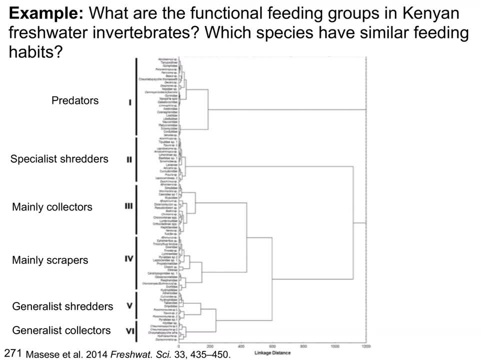 at what the species had eaten and they used this to calculate distances between species, which were then put into cluster analysis to identify groups, and we see here that they came up with some grouping structure based on the feeding of the origin of the of the invertebrates, and that can be helpful in ecological analyzes. 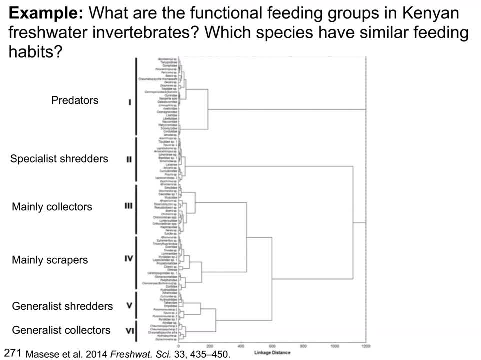 we see that in some of the groups they are relatively succinct and homogeneous. where clusters are built and some are relatively heterogeneous. for example, if you look at the scrapers and compare them to the predators, for example, you see two groups of predators, but within the individual group of predators. if you move to the left you barely see: but there's merging. 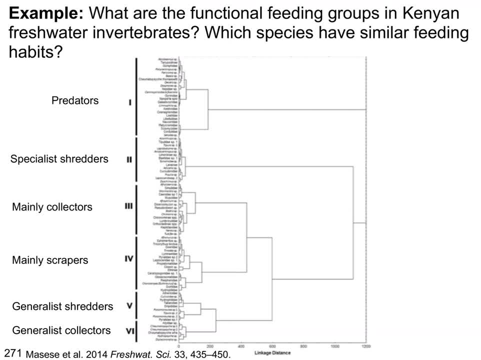 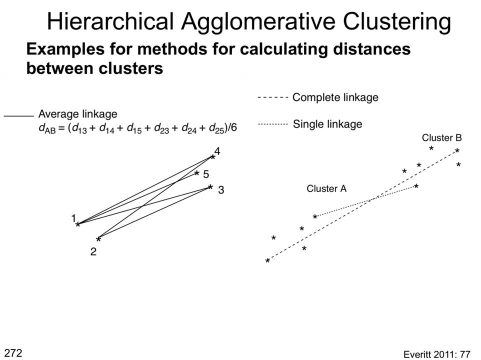 of clusters, so they are fairly similar. you so we have already discussed that one of the challenges in hierarchical acclomerative clustering is that we need to calculate distances between the clusters- orbital in objects and clusters. and how do we do this? and there are three different methods that are applied. this plane on this slide, so on the one. 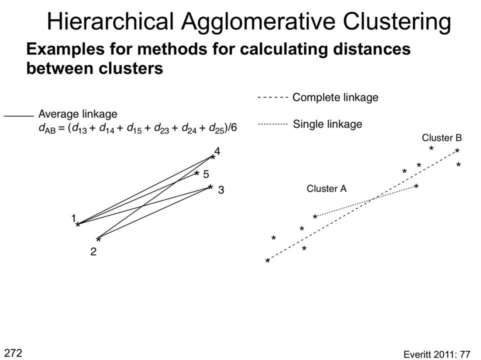 hand you have the average linkage. that means If you have two clusters that are visualized here by- 1 and 2 is seen as one cluster and 4,, 5,, 6 is seen as one cluster- then you take all the distances between 1 and 4, 1 and 5, 1 and 3 and so on and you compare the distances between 2 and 4, 5 and 3 and so on. 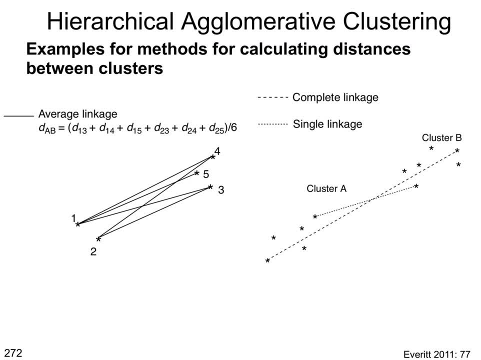 You calculate all individual distances between the points and you take the average, So it's the average distance between all individual objects in the clusters. On the other hand, as you have seen before, we could take the shortest distance between the objects. So if you have a cluster A and B, as shown on the right-hand side, we have a couple objects. 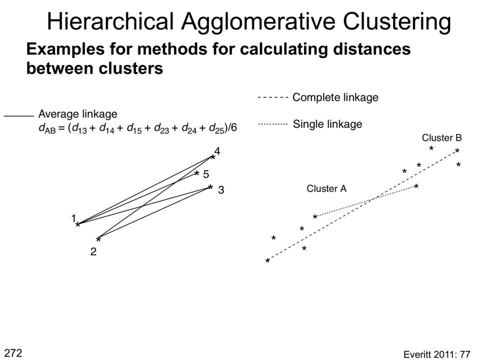 We have a couple of points in each cluster and we take the shortest distance between the two clusters. So the points that have the shortest distances provide the distance between the cluster A and the cluster B. On the other hand, we could also say: well, let's take the points that are most distant between cluster A and cluster B. 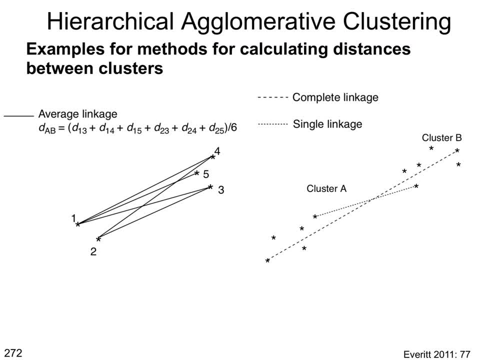 and take this as the distance between clusters. So let's take the shortest distance between cluster A and cluster B and take this as the distance between cluster A and cluster B. That's called complete linkage. Another method is the so-called Ward's method. 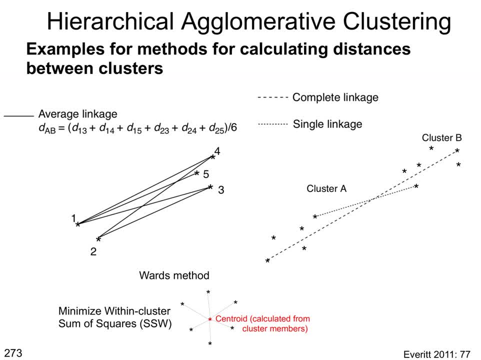 Here we have some similarity to the analysis of variance, because what we do is we try to minimize the width in cluster sum of squares. And how is this calculated? Well, we calculate the center of the individual points in the cluster. so the average. 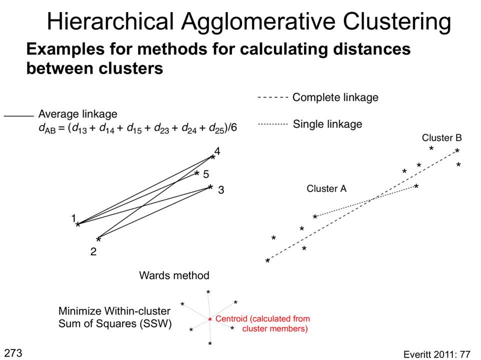 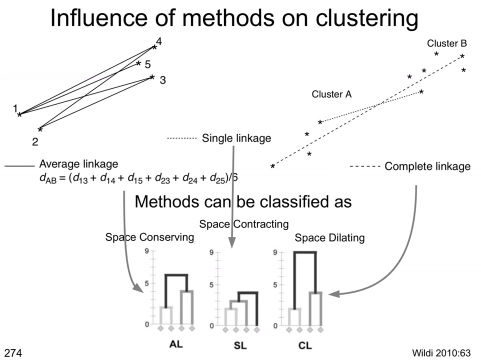 And then we calculate the distance of each individual member from this centroid and square the distances to this centroid and take the sum of this. So you are used to this of doing this from analysis of variance, where you do this for groups. Now, the different methods of clustering have influence on the results of the clustering. 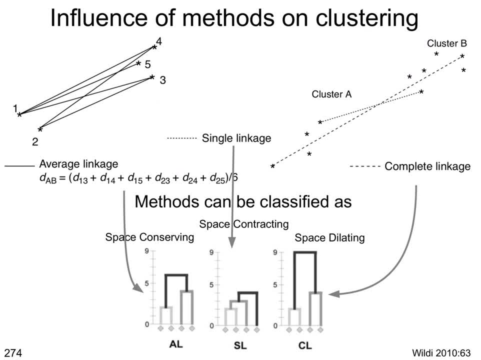 For example, the average linkage is space conserving. The average linkage is space conserving, The single linkage is space contracting And the complete linkage is rather space dilating. What does this mean? Space conserving, space constructing and space dilating. 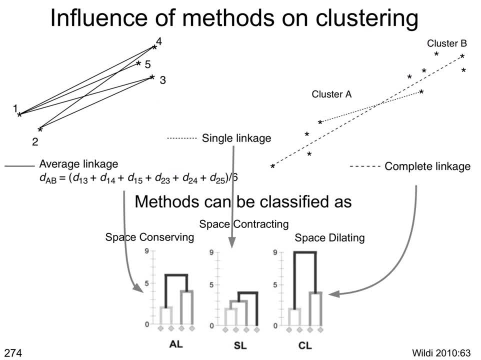 It means, when we look at the original distances between objects and at the distances between objects in the clusters or space conserving matrix, we have a very similar distances between the original distances and the distances after clustering, And we can calculate the distances with the so-called co-finetic matrix. 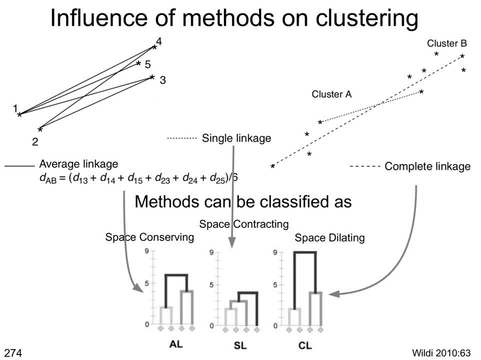 And that's shown to you in R. We can also compute the so-called stress one. We have discussed this metric in the context of NMDS, So go back to the NMDS discussion to see the formula For this goodness of fit measure. 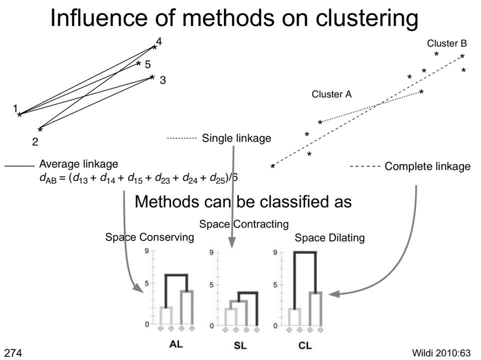 And this would be lower, lowest for the average linkage compared to the single or complete linkage, Because here we have the most similar. we have the highest preservation of conservation of the initial distances. So if we want to preserve the initial distances, then this is the method of choice. 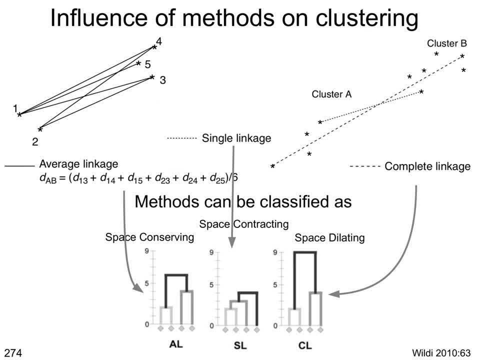 On the other hand, you have space contracting methods. that's used if we want to have very succinct clusters. So this approach adds objects to clusters, even if this leads to shorter distances between clusters than between objects in the raw data. So we aim at building very 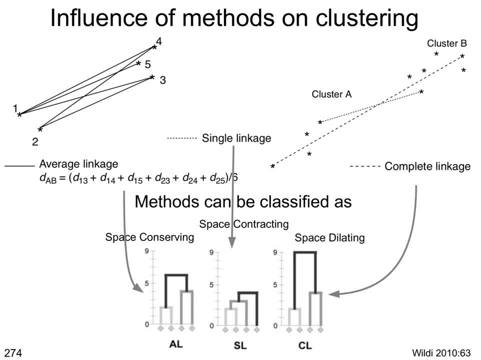 so we would build larger groups, because we add all objects that are close to any of the members in the cluster, And this can be used, for example, to find discontinuities in the data, Because if we have some clusters where all objects are far apart, 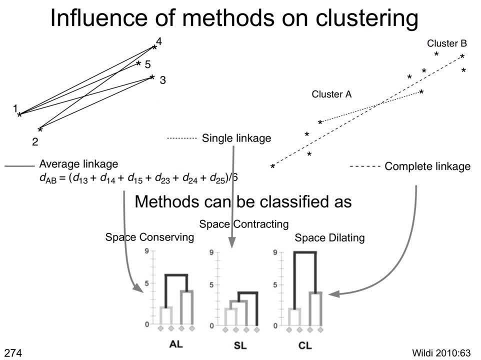 then this can be identified with this method, Because if any of the objects is close to one of the objects in the other cluster, that would be then merged. based on space contracting methods, Space delighting is the exact opposite. This approach minimizes the distances. 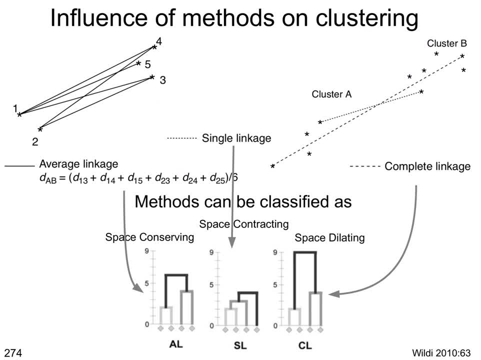 of the objects within the clusters. So clusters are really homogeneous because you always as a distance between two clusters, you always take the distance of the most distant objects, or between two clusters, or a cluster and an object, And this guarantees that only objects. 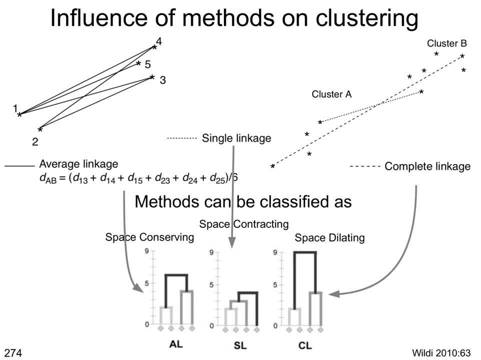 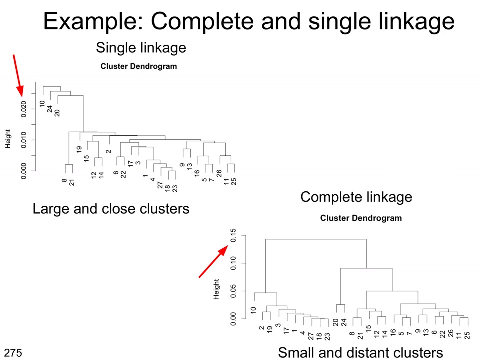 are added to clusters that are very similar to the remaining objects in the cluster. So if you want to find very homogeneous groups in your data, this is the method of choice. So here you see an example where we use some ecological site data. 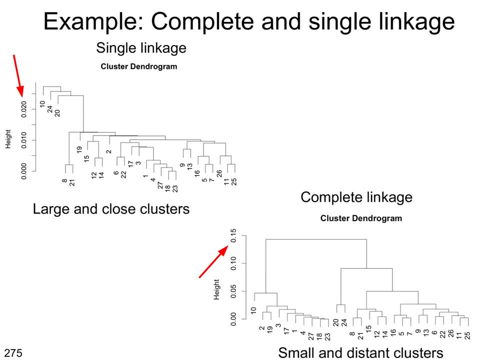 and where some organisms have been measured, and we used two different methods, a single linkage and a complete linkage- to build clusters. What you see is that for the single linkage, relatively quickly look at the y-axis here. That's the distance, It's called height here. 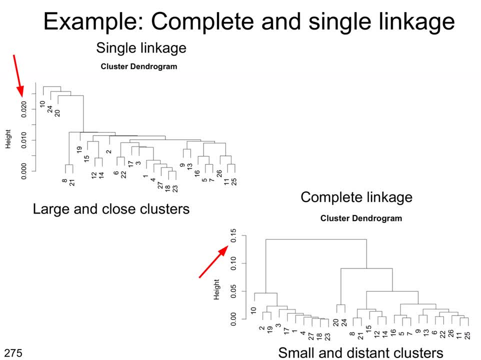 It's the distance between the objects. We see that at a distance of 0.01,. almost always, almost all of the objects have been of the sites have been merged into one cluster And you see that three sites, 10, 24 and 20,. 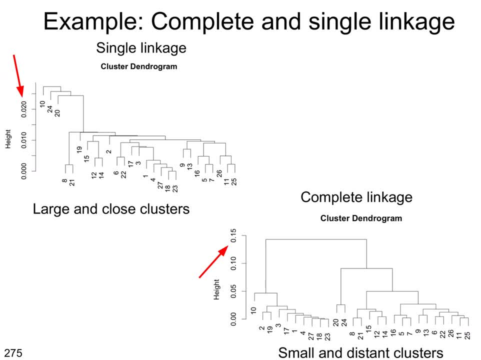 are really different to all the other sites, So you could use this to identify outlines. You could say: well, these are really discontinuous compared to all of the other sites, So you obtain large and close clusters. On the other hand, 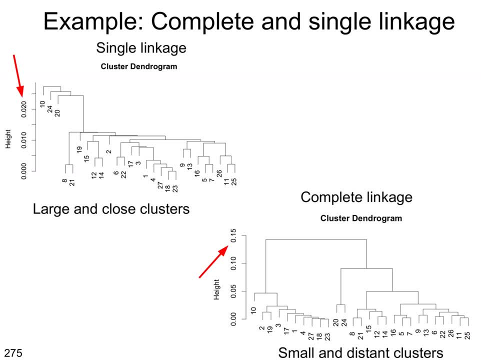 you have complete linkage. It's shown on the bottom figure. Note that we have a very different scale of the y-axis here. So when most objects are merged into a group, we have a tenfold higher distance or height in this dendrogram. 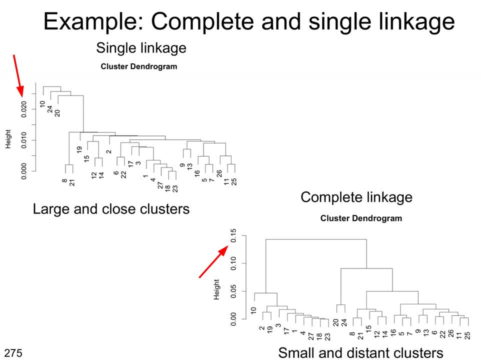 And we see that we have many, many small and more distant clusters that have been established. So if we are more interested in a more homogeneous cluster, then we should take this Note that anyway, we also would identify that 20 and 24,. 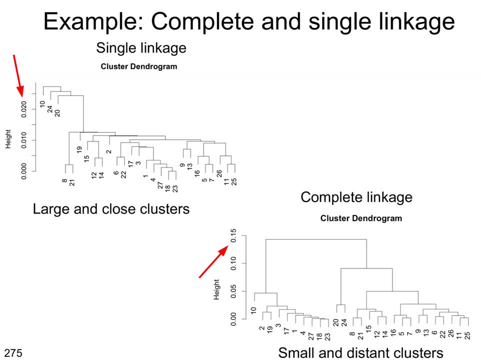 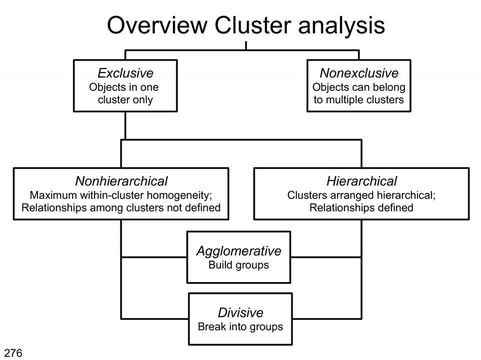 as well as 10, are relatively distant to the other sites In the data set, So there would be some similarity in the results. We have so far discussed hierarchical and agglomerative clustering. Cluster analysis actually consists of many different methods. 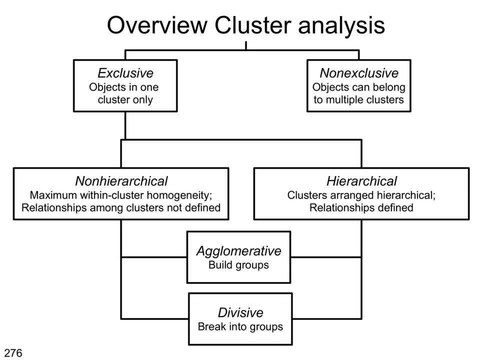 And first you can distinguish. do we place all objects into one cluster only or do we allow objects to be part of multiple clusters? That would be fuzzy clustering. It's called non-exclusive clustering And it's described in Everett et al. 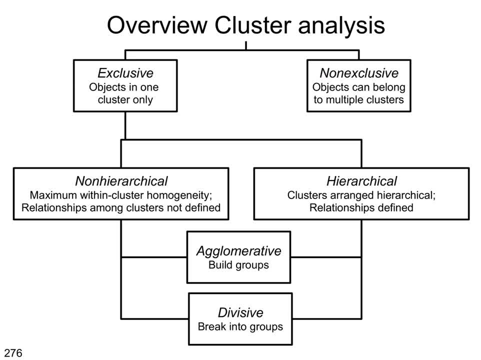 We don't discuss this in detail here. We only go along this line or go along the line of exclusive clustering. that means objects can only be part of one cluster. And then we have non-hierarchical and hierarchical clustering. Hierarchical clustering is clustering where clusters are arranged. 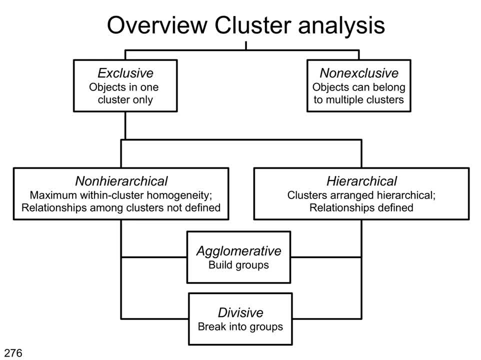 in a stepwise procedure. So you have clusters merged at one stage and in the next step Another cluster is merged, Other objects are merged, So you have the stepwise until at the end all of the objects are part of one big cluster. 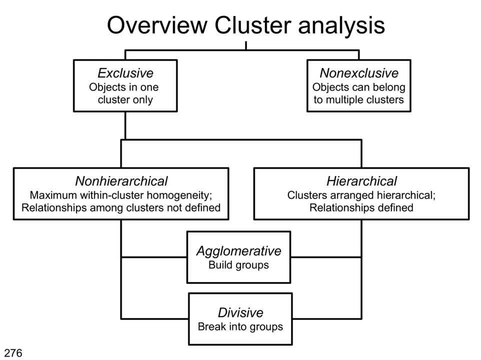 or each has one single cluster. And that's the difference between agglomerative clustering, where you start with each object in one cluster or one group and you merge them, or with hierarchical, divisive clustering, where you would start with one big group and break up into smaller groups. 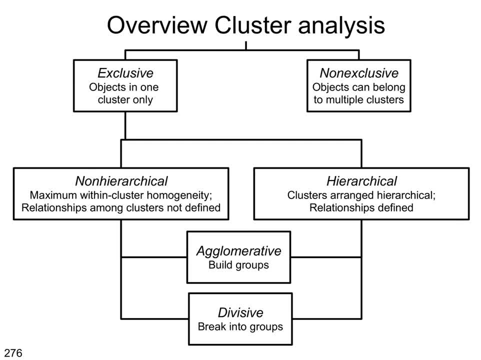 So hierarchical, agglomerative clustering is what we have discussed so far. What we will discuss now, which is different to that, is non-hierarchical clustering, And this is used to look at maximum. It also looks at maximum within cluster homogeneity. 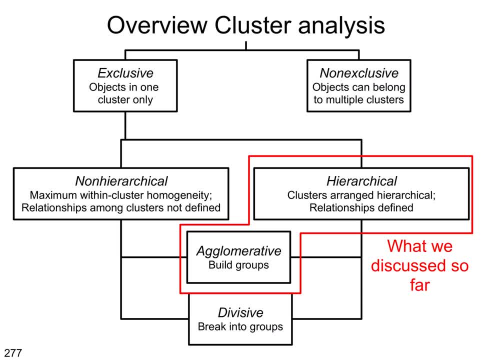 homogeneity, but there is no clear relationship between the cluster. There is no stepwise procedure, So we come up with one partition of the objects in the different clusters, but we don't obtain the steps that led to this result, because the algorithm is very different. 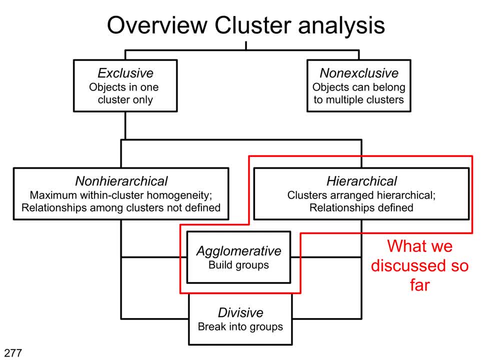 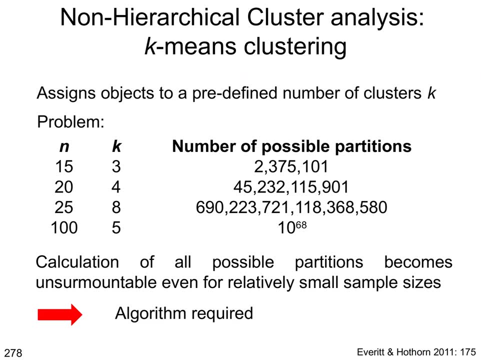 So we don't have a stepwise procedure here. We will discuss when you should use what after we have discussed k-means or non-hierarchical cluster analysis. So non-hierarchical cluster analysis. there are different types, the most or different methods. 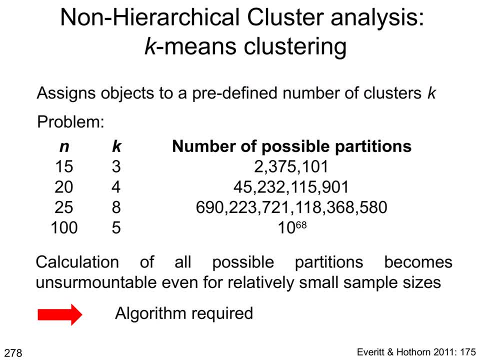 And the most widespread one is the k-means clustering. It's not necessarily the best one, but if you understand that, you will understand its descendants that have been developed later on. We will show you later, on one of the slides, some additional techniques. 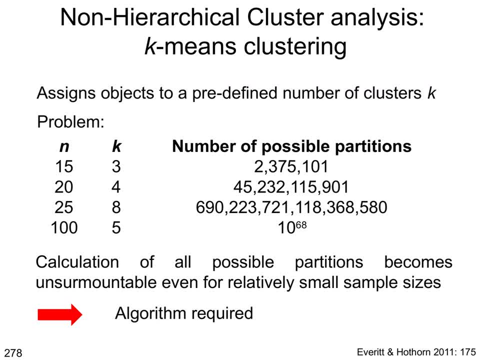 that can be used if you have different problems or research questions that cannot be answered by k-means clustering, So it assigns objects to a predefined number of clusters. So that's very different to the previous clustering method. In the previous clustering method 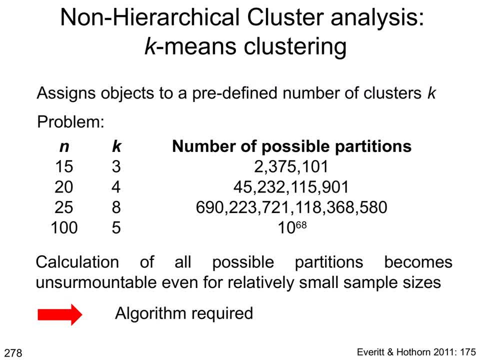 we could cut this hierarchical tree wherever we want and then have a number of clusters that we wish to have. Here we assign objects to a predefined number of clusters, So we need to define before that we want to have three groups or four groups. 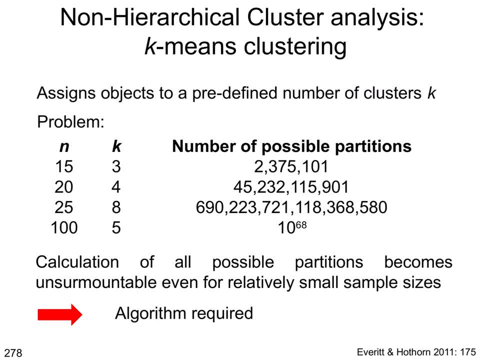 or five groups or whatever. And that is the problem, because if in the example here some numbers are given, if we have, for example, 15 objects and partition them between three groups, there are already two million different possible partitions. Now if we have a sample size of 100,. 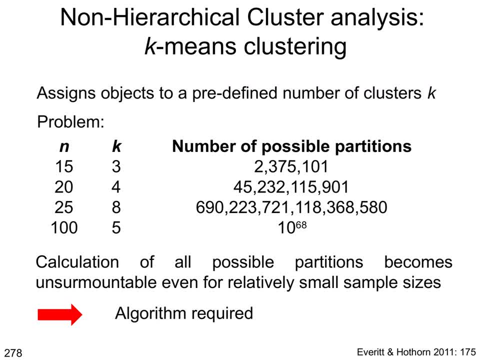 which is not unlikely. so you often have 100 samples and you have all five groups. then the number of possible partitions becomes incredibly large. So we cannot calculate all possible partitions. This becomes unsurmountable even for relatively small sample size. So we need an algorithm. 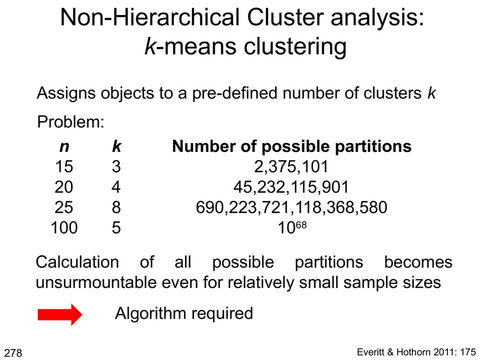 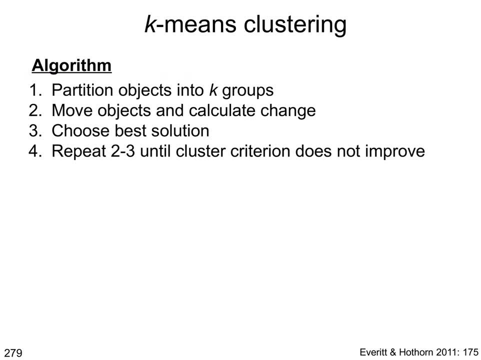 that does this for us and finds a solution or an alternative to calculating all possible partitions. So we need an algorithm that helps us to find a solution to this problem, And this algorithm, in the k-means clustering, is outlined here. We first partition all objects. 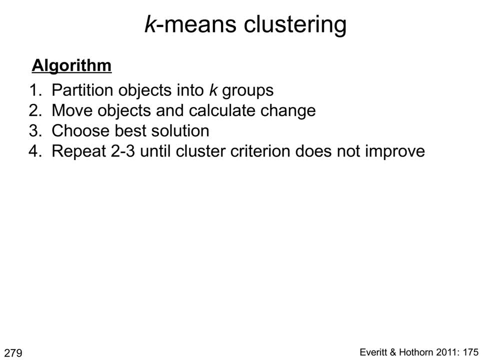 into k groups. then we move objects between groups and calculate a change in a cluster criterion. Then we compare the cluster criterion between the initial situation and the situation after we move the object. So we calculate whether the change improved or decreased the quality of the cluster criterion. 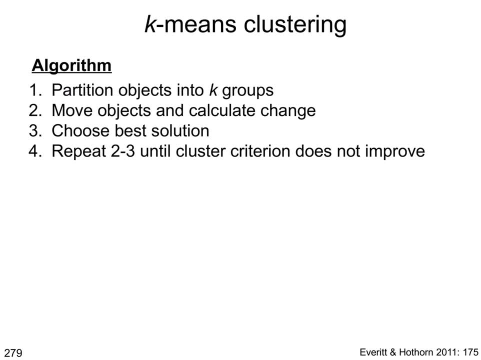 and repeat this until we have no visible change anymore in the cluster criterion. So we need to have a criterion that tells us does the clustering become better or does it become worse when we put place points in different clusters. So it's clear that this 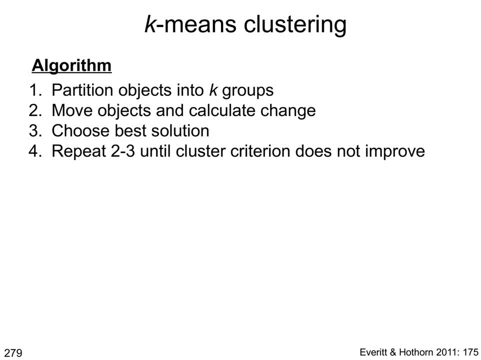 given the waste amount of possible partitions, it's clear that we don't find the best solution necessarily if we just start with one type of assignment of objects in two different groups. So we need another, So the algorithm needs to be started multiple times. 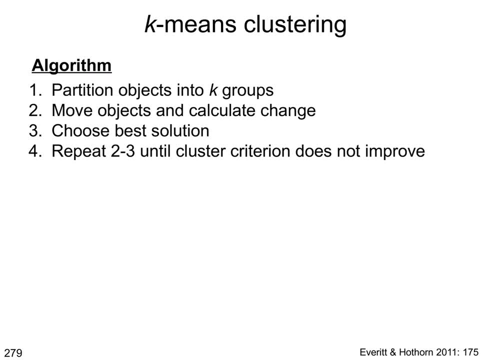 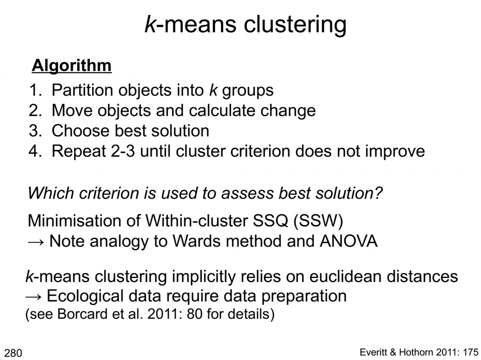 with a random partitioning into the desired number of groups. In fact, you could also use a non-random partitioning, For example the result of a hierarchical cluster analysis, as a starting point. So which criterion can be used to assess what is the best solution? 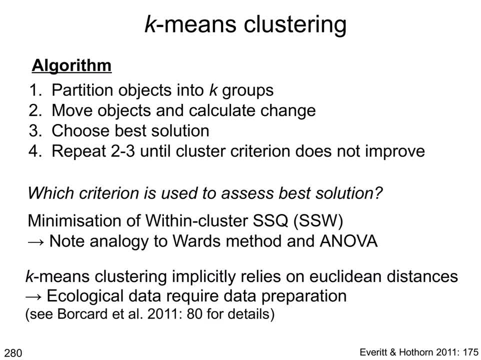 and to assess how change affects the clustering. Well, that's again the minimization of the width in cluster sum of squares. So we want to have to move objects into one cluster that are very similar, that have a low distance, and this distance is measured. 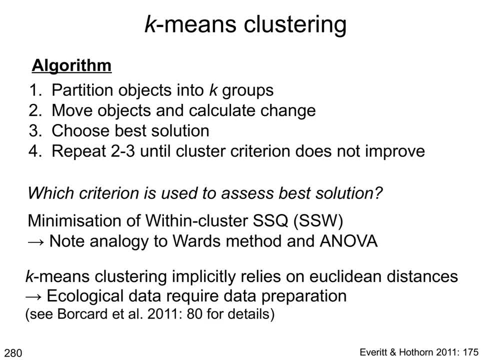 of the sum of squares within clusters And note here the analogy to the Ward's method in hierarchical and non-acclomerative clustering and to analysis of variance that I mentioned before in the context. Ward's method K-means clustering implicitly relies on the Euclidean distances. 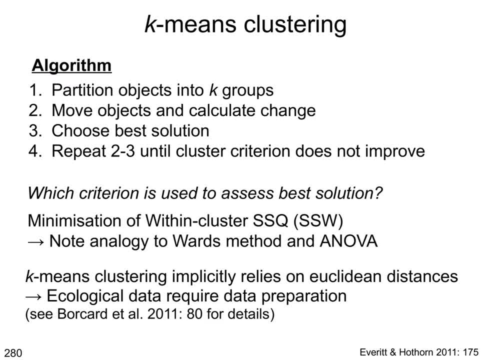 when the sum of squares are calculated. So if you want to use it for ecological data, this requires some data preparation, For example, transformation of the data so that the Euclidean distance can be used. with that We discussed the problems of the Euclidean distance. 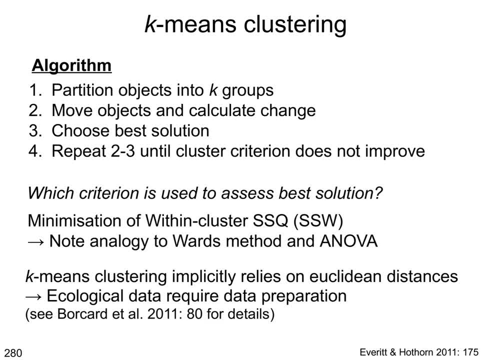 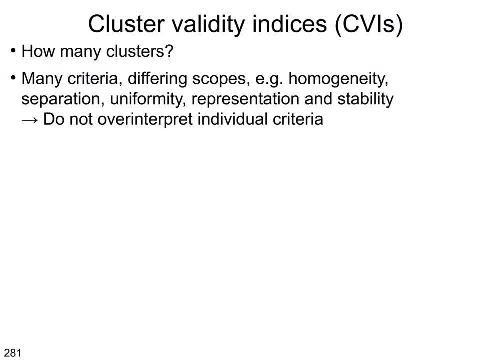 for the ecological data in a previous lecture on similarity measures. Now, after that, we have done all the clustering, either with K-means or with the hierarchical and non-acclomerative clustering. one question certainly remains, and that is: how many clusters do we really have? 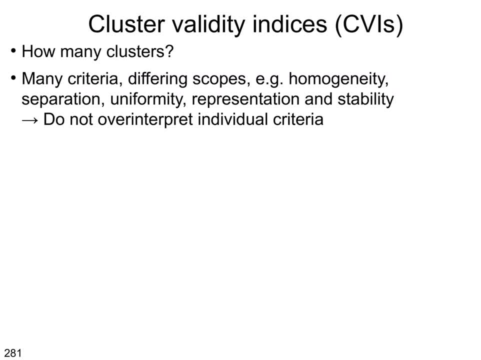 So we could, if you imagine, a study where we had observed the different sites and the environmental variables like pH, temperature and nutrient concentrations and so on. in the sites we could run on hierarchical and non-acclomerative clustering that would show us in a dendrogram. 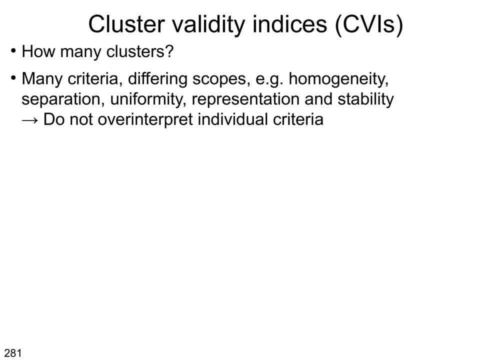 how the different objects are merged. but in the end they are all merged into one cluster. and where do we draw the line? Where do we say: well, that's the number of clusters that we want to have? We could do this visually looking at the dendrogram. 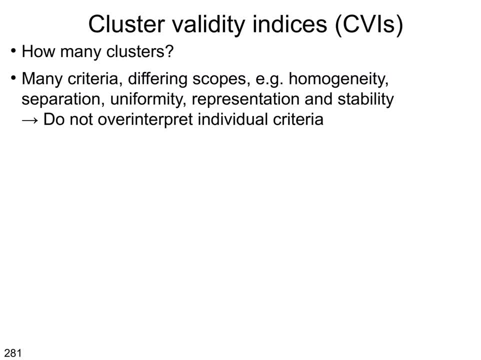 for a K-means clustering it's even different. We have to provide a number of clusters before. But what is a good number of clusters? Is it 4, 5, 10, 20?? So we need to have a criterion. 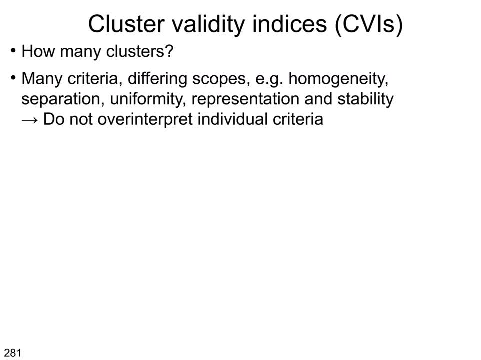 and these are called cluster validity indices. that allows us to compare the validity of the clustering between different number of clusters. Now you can imagine that there is a wide range of criteria again and we can't go into all details of these individual criteria here. 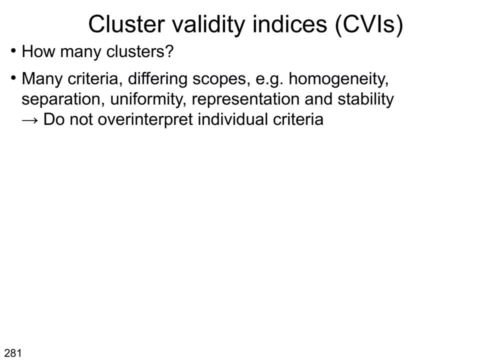 Just, you should be aware that these criteria- there is no one size fits all distribution- but they have different scopes. One are better to evaluate homogeneity of the clusters. other put more weight on the separation between clusters. others look at uniformity of the different clusters, so that you 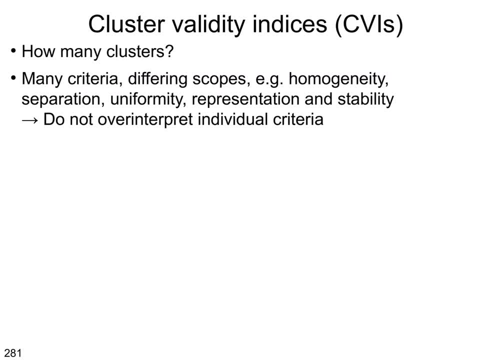 have clusters that are relatively uniform in their homogeneity or separation, Then some of these criteria are the representation of the raw data and others the stability. So how stable is the solution if you have change, if you had changes in the raw data, You should 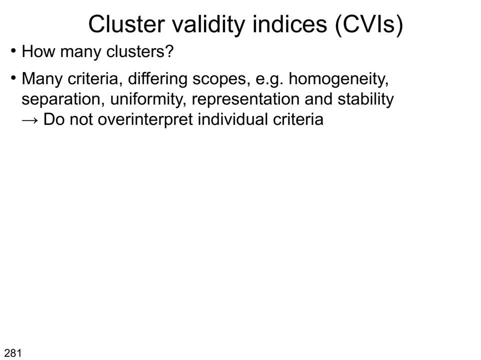 not over interpret individual criteria and be aware that all of these criteria are based on the data that you have in the data. So you should not over interpret the data that you have in the data. So you should not over interpret the data that. 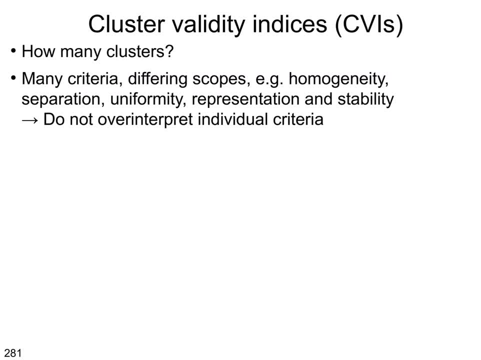 you have in the data. So you should not over interpret the data that you have in the data. Then you should not over interpret the. We could check whether the grouping structure that we have externally given- for example, sites in the forest and agriculture and urban landscapes- resembles the resulting cluster structure. 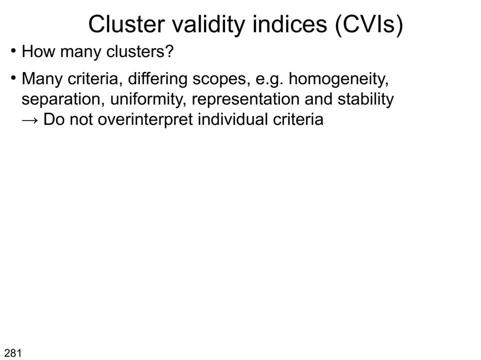 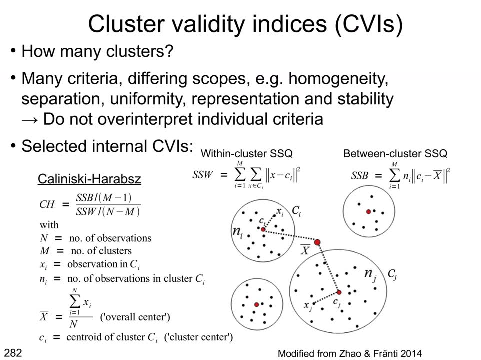 These CVIs that I used here are so-called external CVIs. Now we discuss the first internal CVI. This index is called Saliniski-Harabsch. This index, calc, is similar to ANOVA. Remember that in ANOVA you calculate the sum of squares within and the sum of squares between. 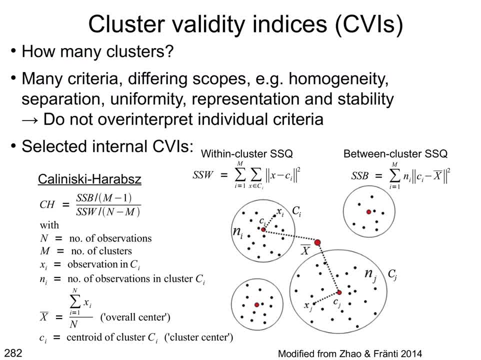 And this is similar in this index. If you look at the picture you see, or in the figure, the right bottom, you see four clusters. Each of the clusters has a C. Ci is the cluster on the top left, Cj is the cluster on the bottom right. 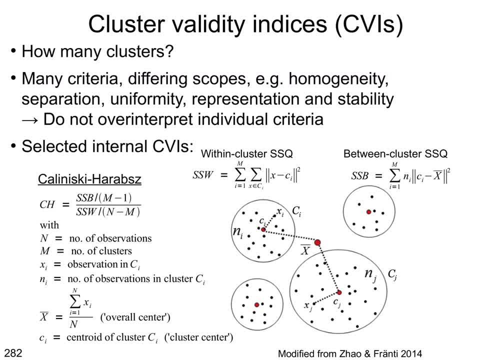 Then you see an X with an overline and this indicates the total mean of all data. That's the right point in the center, and then you see red points within each cluster. These are the centroids, That's the lower C that indicates these points, and the number of points in each cluster is N, so the number of observations. 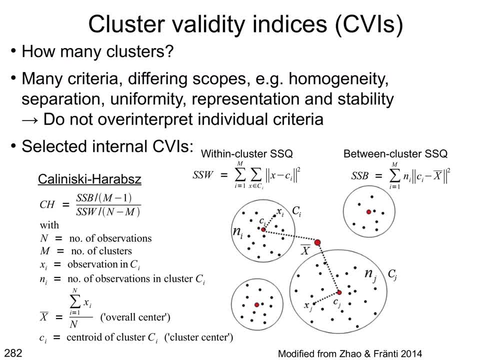 Now what you do, and without going too much into details of the few formulas for calculating the Saliniski-Harabsch index, the CH index, which we will just refer to in the following, is you calculate the within clusters sum of squares. 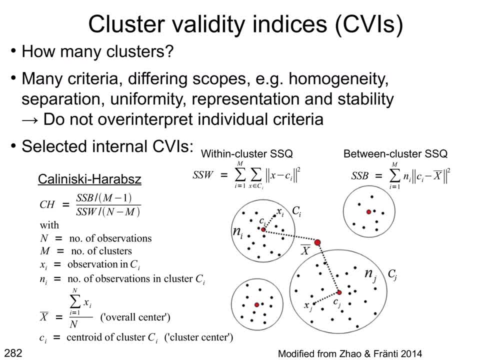 So you take each observation and you calculate the distance to the centroid within each cluster and this will then be squared, and you calculate the sum between clusters And for that you take the center of all data, which is indicated by the x over line in the red point, in the center of all clusters. 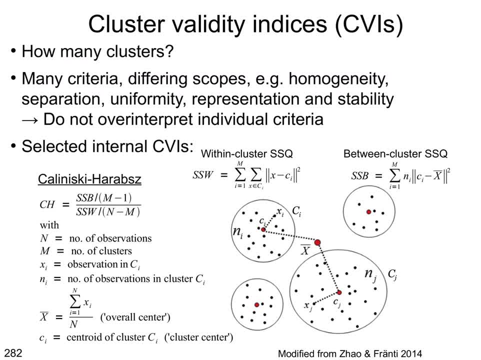 And you calculate the distance from this one to all observations. And then you have the formula where you divide the between cluster sum of squares by the within cluster sum of squares. And it should be quite obvious what is that, how the goodness of fit is indicated. 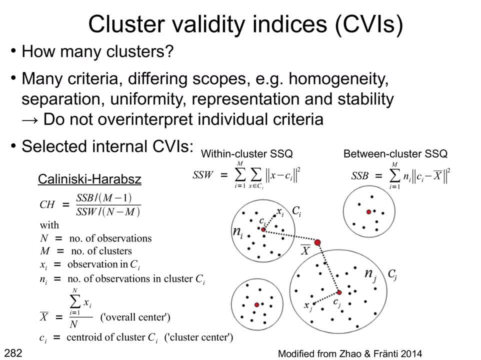 It's clear that the higher the CH index the better the clustering is. then Because the clustering you want to minimize the within cluster sum of squares and you want to maximize the between cluster sum of squares. So a higher Salinitsky-Harapsch index is better. 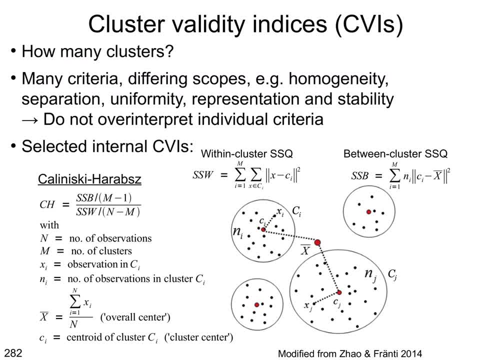 So that means, if you calculate this index for a couple of for different cluster solutions, let's say one one for for hierarchical clustering you have four, five, six or seven. or for k-means you have four, five, six, seven groups selected- Then you can compare these groups with the CH. 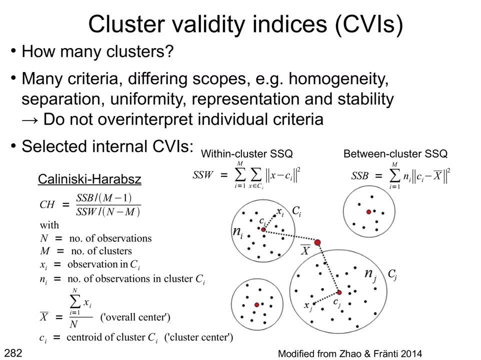 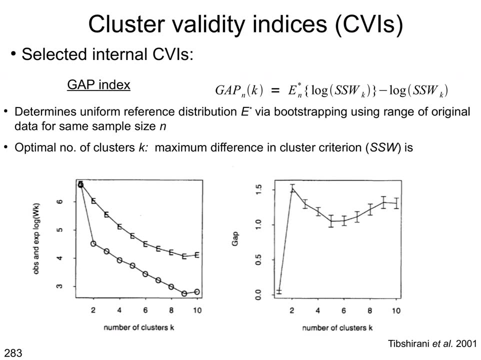 index and you would select the group that shows the maximum CH, So the number of groups that shows the maximum CH. An index that follows a different approach is the so-called gap index. It's also an internal CVI And, while this looks- again based on the formula, a little bit difficult, 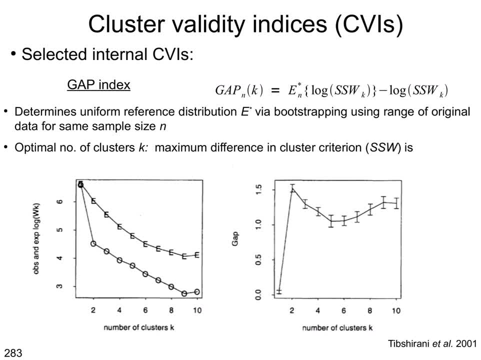 you have that. it's actually quite simple. What it does is it calculates the different reference in the sum of squares within clusters, so SSV between the data and between the reference distribution. That means that initially, what the algorithm does, that calculates its index. 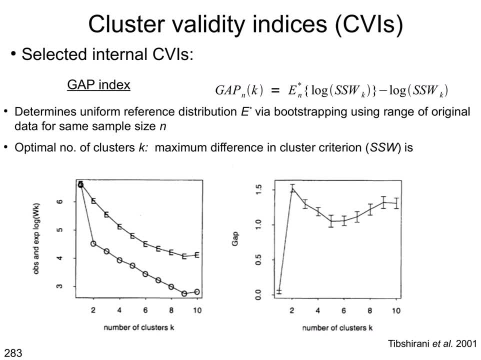 it determines a uniform reference distribution via bootstraping, So it doesn't assume a particular normal distribution or whatever, but every value within the range of the data, of the original data, has the same probability of being selected. That's a uniform distribution. Normal distribution would have a mean and the further 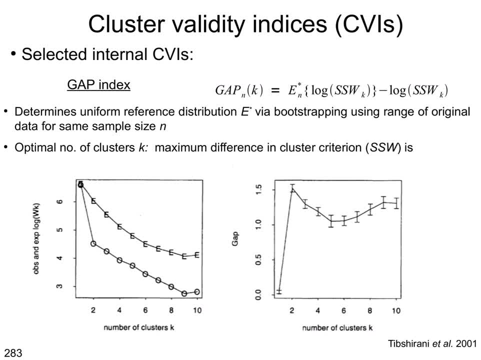 you are away from the mean, the lower the probability would be to be selected as a value. So, with this uniform distribution, you calculate as well the sum of squares within for the clustering and you compare the results between these pure random data and between the data that originates. 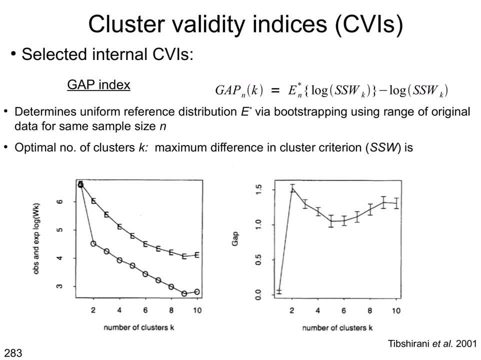 or the clustering that originates from your original data And what you can see is in the figures below: if you plot the observation, the number of clusters of the observations and the sum of squares within and for the reference distribution, E that you have a difference between these, both between the values for the reference, 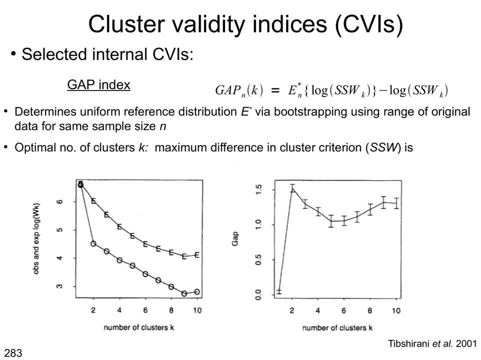 distribution and for the original data. For example, if we look at four clusters and the left bottom plot, you see that the log of the within cluster sum of squares is about four, but the log for the reference distribution clustering is about five. So there's one. 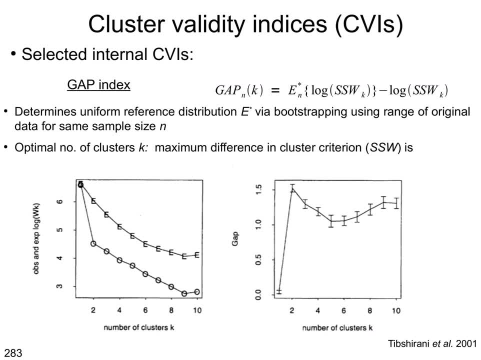 one log unit difference between them And what we now look for. we search for the pair of observation and reference distribution data that has the highest difference, And this is actually shown on the right hand side, where you see that the strongest distance is given for two clusters. 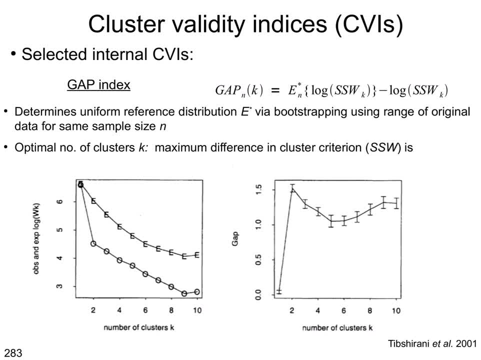 and so that's the 1.5 log units difference in between the uniform random distribution and between the original data. And yeah, you would select two clusters in this case because you have the highest gap value, the highest distance between this reference distribution and the original data. 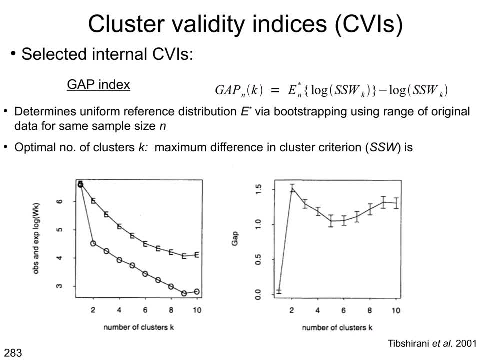 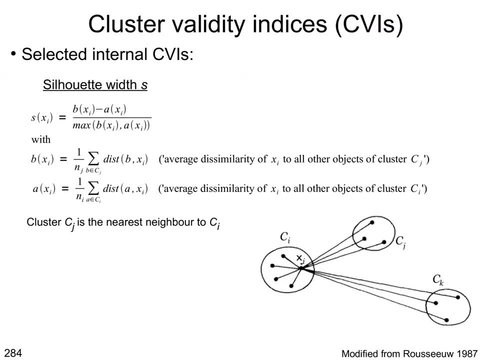 clustering, And now you can actually crack down on one cluster on the other and from that you will just see the number of clusters that have the highest difference between these two. Another internal CVI is the silhouette width, and this relies on the dissimilarities of an observation. 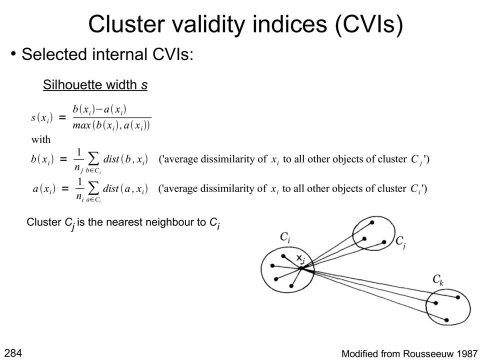 to, or the dissimilarity of an observation to, the other objects in the same cluster, compared to the average dissimilarity of the average similarity of the objects within one cluster and the quantity of 85 to the other objects within one cluster. So we can write down here the average dissimilarity of the 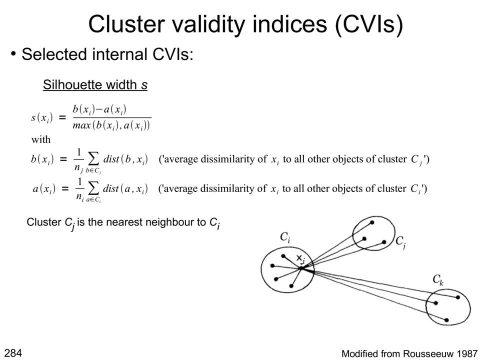 of objects in the nearest neighbor cluster, So just indicated by the figure below, you take an observation, xe, and you calculate, within the same cluster, the similarity, the distances, and take the average of that one and you do the same in this case. 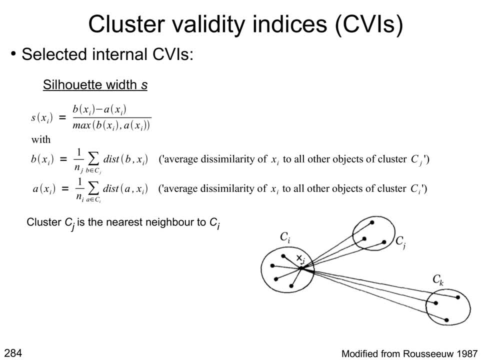 the nearest neighboring cluster would be cj. you calculate for xy xe the distances to the individual points in the cluster cj and take the average. And it's somehow obvious that if the average dissimilarity with clusters, with their own cluster, is higher than the average dissimilarity, 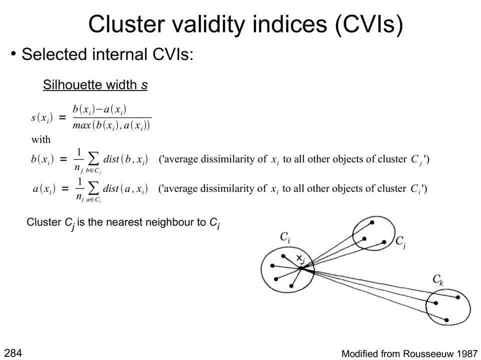 to clusters, to another cluster, then it would be better to actually place that dissimilarity on these observations in a different cluster. So ideally, all of the silhouette width would be larger than zero, because if it's smaller than zero means based on the formula. 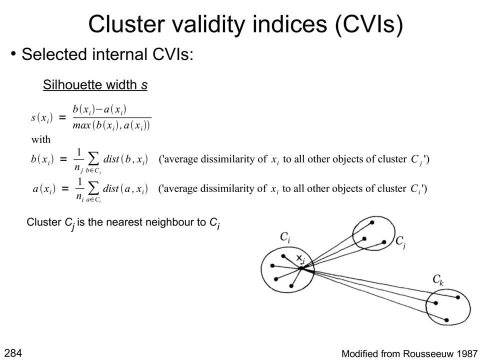 based on that, the average dissimilarity with the observations in your own cluster is higher than dissimilarity with observations from others, another cluster, and this is expressed in the equation that you see here, and the denominator and the equation scales the value and it's relatively similar if we 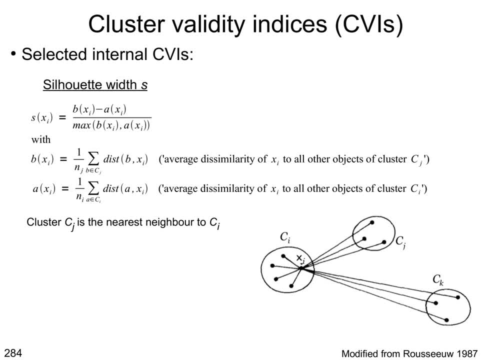 compare it to the Precursor distance how the scaling is done with the maximum here. we want- don't want to go into more details here of the equation you. so what represents good silhouette width for an individual point has already been mentioned. if the point approaches one, it's very well classified it approach if 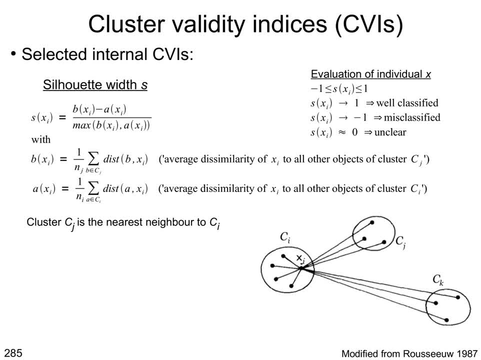 it approaches minus one, it's, it is misclassified. and if it's around zero silhouette width for a point, then it's unclear where this point should be placed. Now, if you don't want to typically, you don't want only to evaluate the results for an individual point. 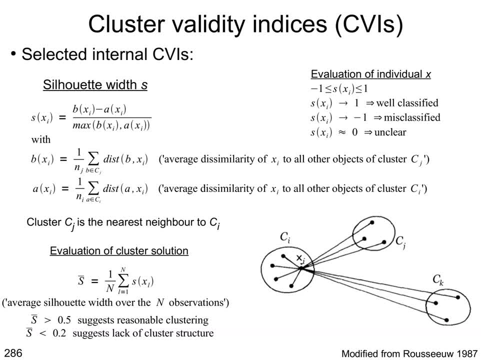 but for the whole cluster solution. if you're using, for example, different number of clusters, you want to compare them and that's where you can use the average silhouette width, And if you use this index, you calculate the average of all silhouette width over the observations. 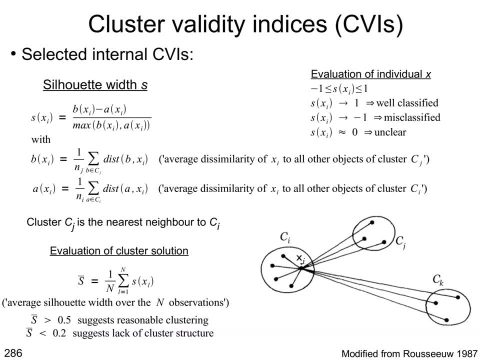 and the higher this silhouette width becomes, the better the clustering is according to this index. So you would select the number of clusters that yield to the highest number for S for the average silhouette width, And if this absolute value of the silhouette width is above 0.5,. 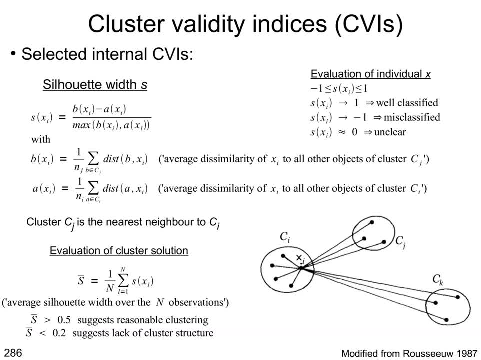 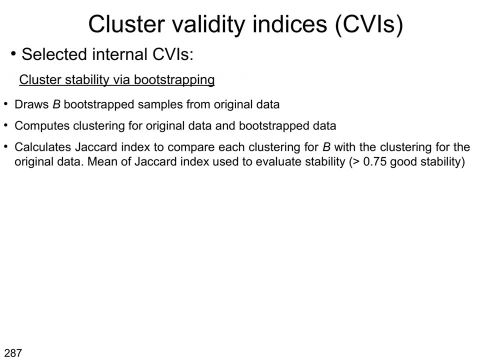 this suggests that you have a reasonable clustering. If the value is below 0.2, this actually would suggest that there is a lack of cluster structure. Finally, a concept that you have visited before is bootstrapping, And bootstrapping can be used to assess the cluster stability. 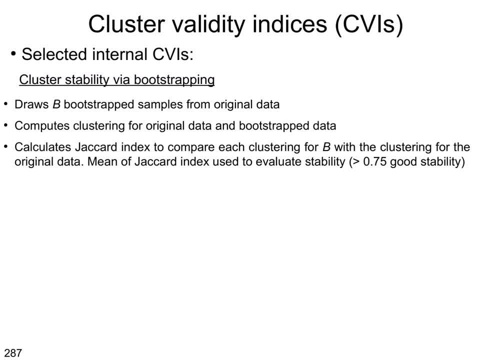 So what you do is you draw bootstrap samples for the original data, So you create 100 additional samples, for example. Then you compute the clustering for the original data and for the bootstrap data, So that follows approximately a similar distribution as the original data. 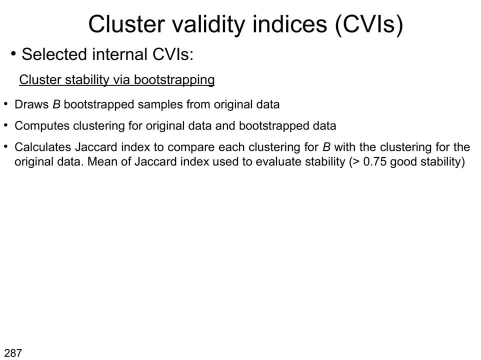 And then you calculate the Jaccard index. So the Jaccard index can be used. You know it's an index for presence absence data And this is actually in this case: you have a presence or a 1, is used if you have the same cluster solution. 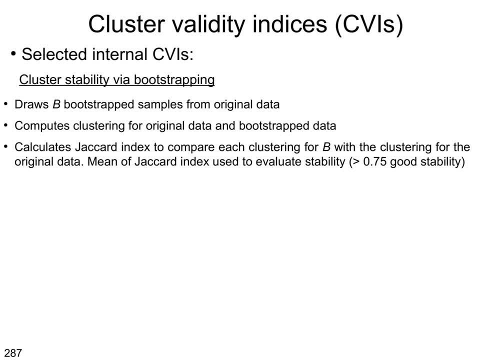 for the original data and the bootstrap data, And if the observations are placed in different clusters, then this yields to a zero, And to evaluate the overall cluster stability, the mean of Jaccard index across all pairs of original data and bootstrap data can be used. 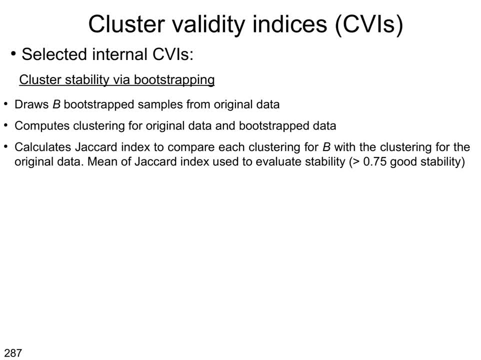 If this mean of the Jaccard index is higher than 0.0, 0.0, 0.75,, then this can be regarded as a good stability. If it's lower, it may be less stable, but this will also depend on the sample size. 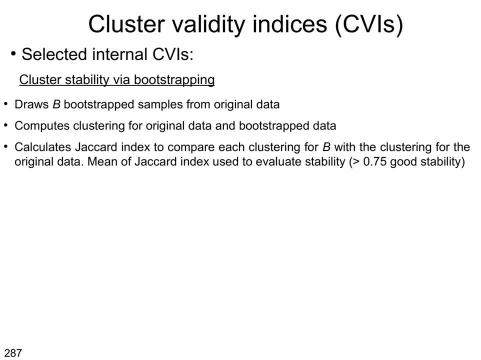 as you will see in the R-Script. So with a larger sample size it's easier to obtain stable clustering than with a lower sample size. But it's also obvious because if you just move one individual point point and this has a stronger effect if you have a few samples than you have many samples. 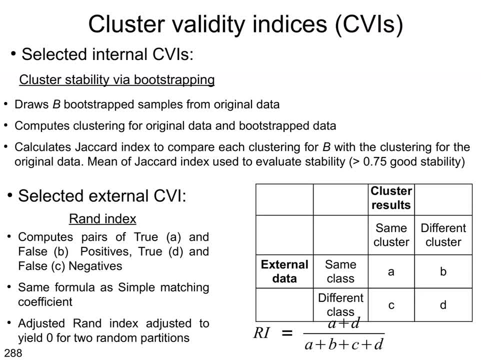 And the final index is an external CVI. so assume that we have a grouping structure that is known beforehand So we can use this to compare the result of our clustering to the external grouping structure, to the external data that is provided. And when you look at the index, the so-called Rand index, the index is the same as the simple. 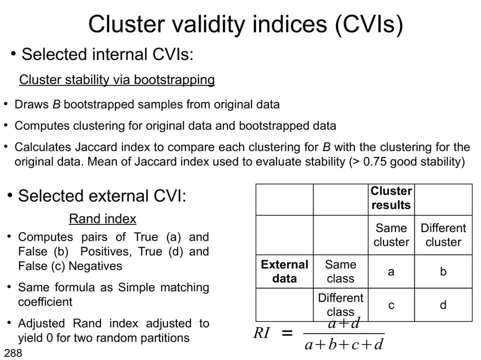 matching coefficient that we had when we discussed similarity. so the same number of measures and distance measures in the previous session. So there's nothing new here. You see also the table has just been adjusted. Instead of species presence, absence, we look at cluster results. 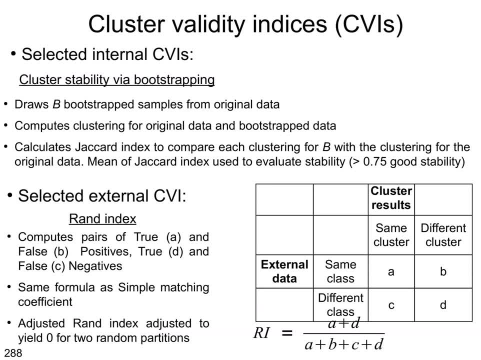 and external data. So you have the a if you have the same class in the external data and it's placed in the same cluster in the cluster results If a pair is placed in a different class in the external data and in a different cluster for the clustering. 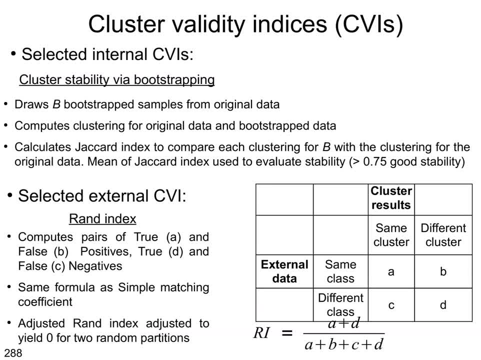 results. it's d, so these are the true positives and the true negatives, And then of course you have also false positives and false negatives. There's also an adjusted Rand index that's adjusted to yield zero for two random partitions. So that's what we use in the R software, but for us it doesn't matter here. 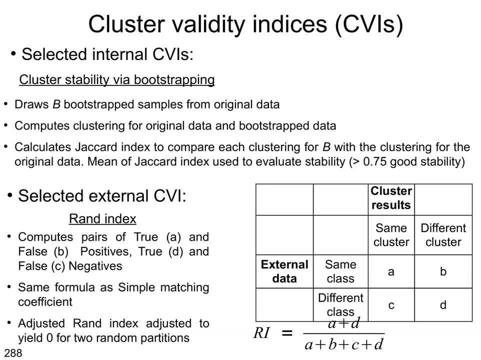 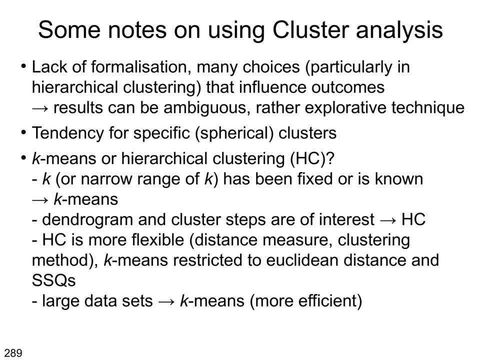 how this more complicated index is calculated. So finally, some notes on using cluster analysis. You may have realized that cluster analysis remains, at least partially, subjective and that there are many different choices that can be used or even be misused. It's certainly a valuable tool for 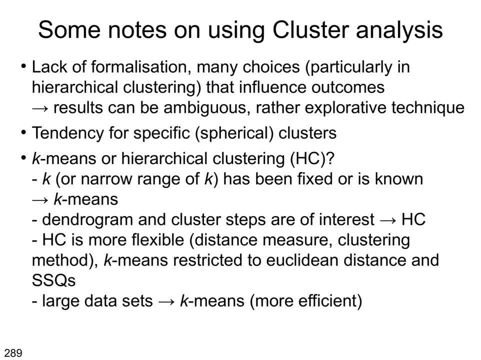 exploratory analysis in different fields, but it lacks formalization, So there is no clear guideline what to do and for different data sets. different approaches or methods may come to better solutions and different choices. For example, the methods associated with hierarchical clustering influence the outcome and it depends 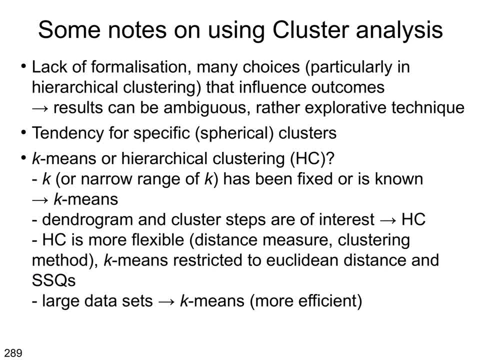 always on the research question. You can also, when you look at the examples that we deal with in the R demonstration, you will see that the results are often not that straightforward. So it's a rather exploratory, explorative technique you use rarely or, depending on the data set you 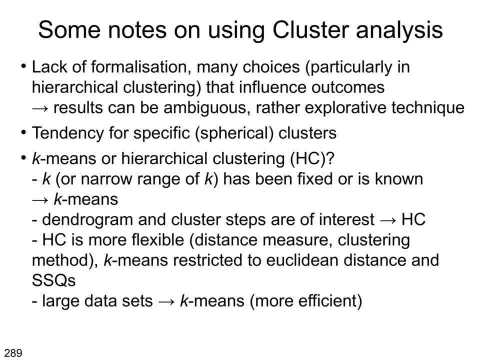 cannot expect to come to really clear solution with different if you would compare the solutions for different methods and for different clustering and you see. so it really depends on your research question, on your aim and what you want to do. It generally has a tendency to detect. 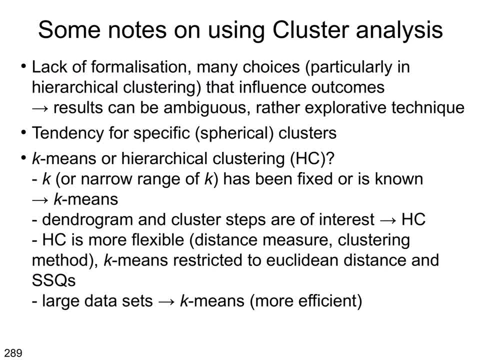 specific kind of clusters or spherical clusters. Some other clusters may not that easily be detected. well, and you might might ask when should you use k-means and when should you use hierarchical clustering? Well, as a few general comments on this choice, k or a narrow k range of k. 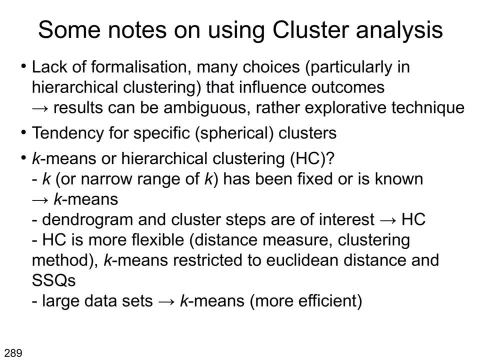 if this is known. so if you know there are few groups in the data and you can narrow this range down, then you should use k-means if you really have knowledge on this. So, for example, let's say we have obtained remote sensing data from the from some. 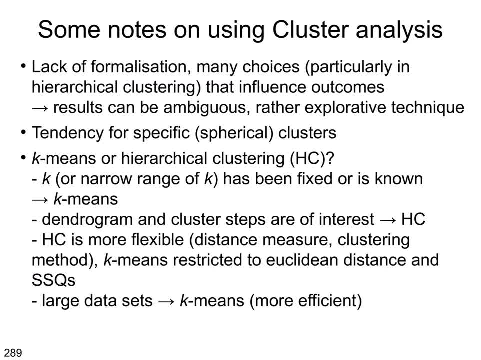 satellite mission on the earth surface and we want to classify the land cover in different land cover classes, then we might know beforehand and we want to have 10 different classes and we can use this for selecting the group. so the group assignment in k-means. On the other hand, if we want to see how the cluster steps, how 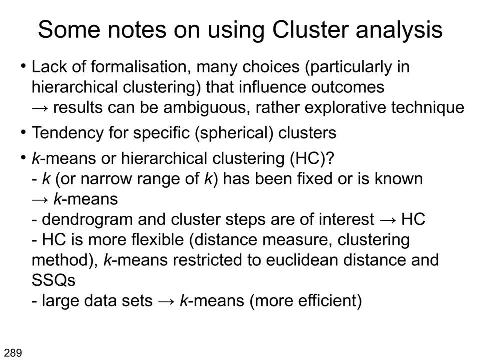 the clustering is done in a stepwise procedure, because we're interested in the pairwise comparison of objects and how these are merged along the clustering and we want to visualize the clustering in the dendrogram. yeah then we should surely use the hierarchic clustering. The hierarchical clustering is also generally more flexible, so it allows the use of different 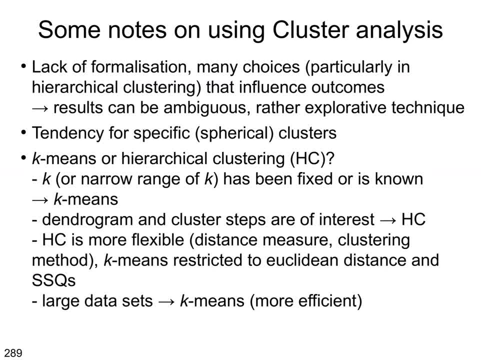 distance measures and different clustering methods, whereas k-means is restricted to the euclidean distance and to the sum of squares. However, there is an alternative to k-means that that we will see. that we will see in the next slide. that is a little bit more versatile than k-means itself. 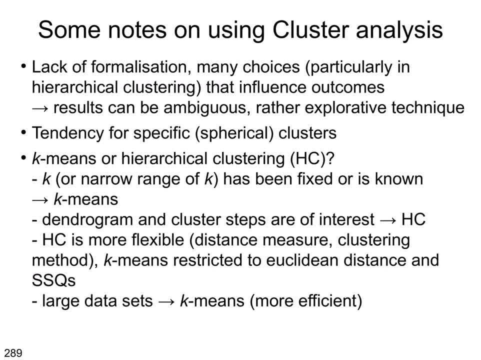 If you have very, very large data sets with 10 000- 100 000 millions of entries, then k-means is actually much more efficient in computation and hierarchical clustering may take too long for computation. I want to end with a quote from Everett et al that you will also find in the note to the slide. 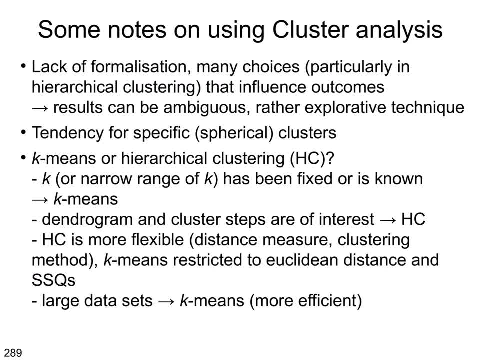 the methods of cluster analysis can be a valuable tool in the exploration of data. Applying the methods in practice, however, requires considerable care if over interpretation is to be avoided. Simply applying a particular particular method of cluster analysis and accepting the solution at face value is, in general, not adequate.